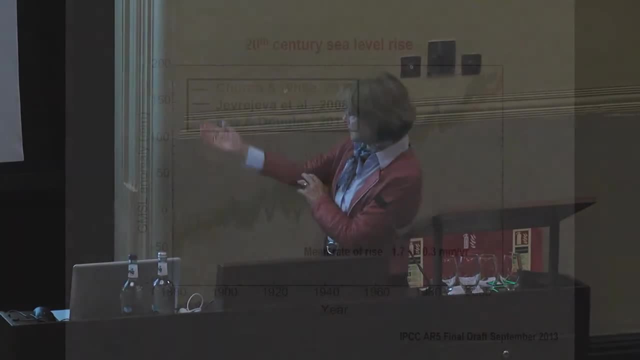 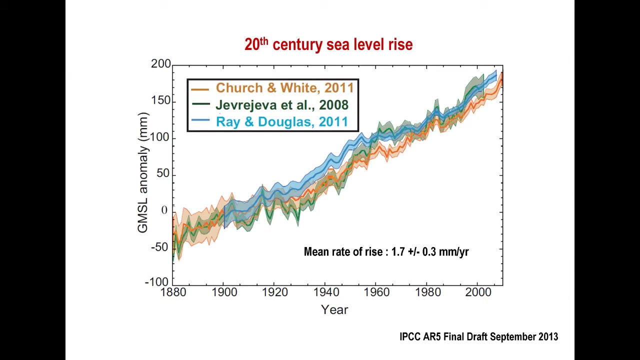 Okay, So let me start with this figure, which is from the IPCC report, and this is a well-known. Is there a pointer? Do you have a pointer? So it is a well-known C-level curve for the last century with different groups from different groups: Church and White, Zhevojeva and co-workers, and Ray and Douglas. 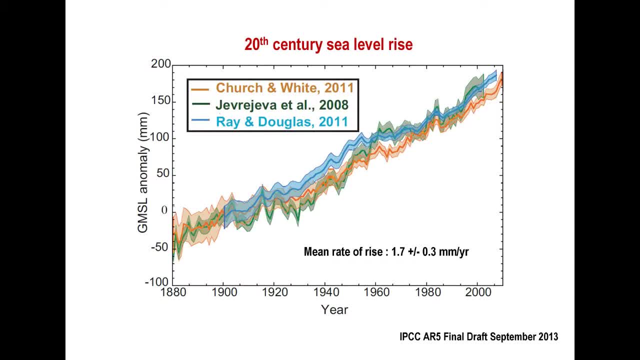 There are others, but Oh, thank you very much. Thank you, Okay. So, as you can see, there are some differences on decadal and interannual time scale, but on average the trend is the same and the mean trend from all data sets gives a rate for the last century of 0.7 plus or minus 0.3 mm per year. 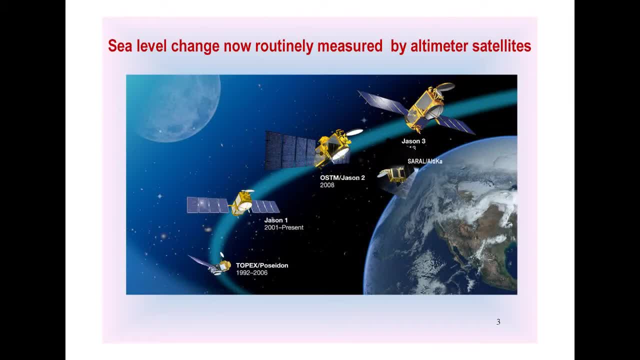 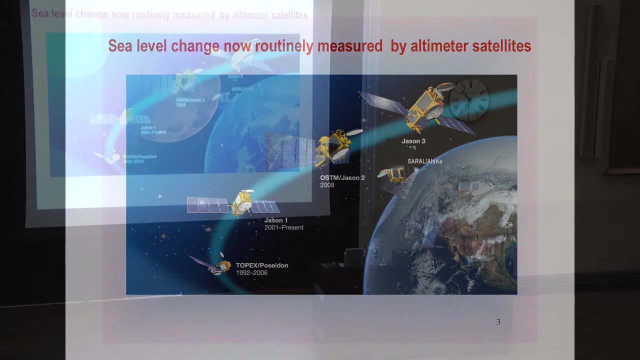 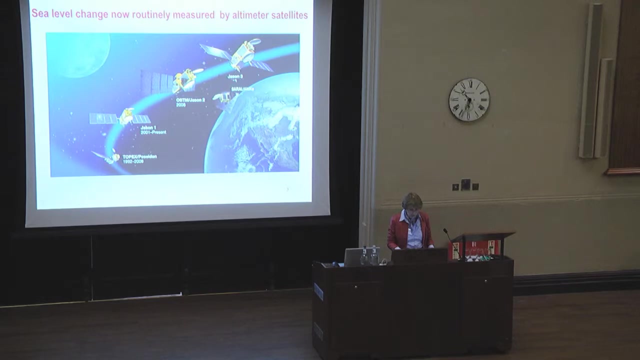 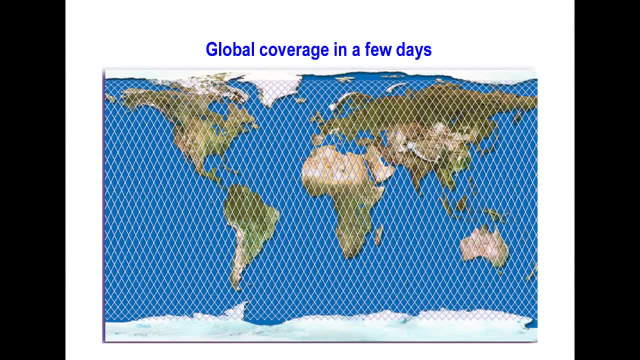 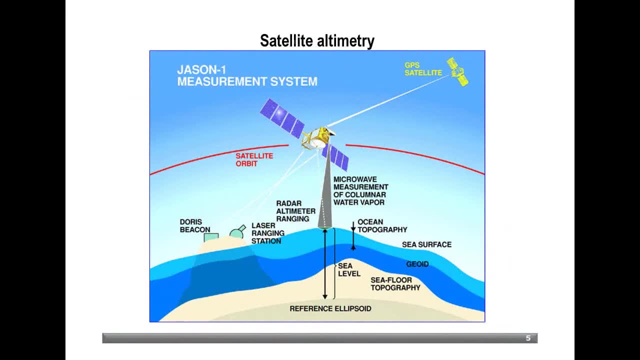 The advantage of satellite altimetry is, of course, the global coverage of the oceans and also the fact that it measures the absolute C-level in a geocentric reference frame, But it does not replace tide gauge, of course. Tide gauge observation is just complementary and both tide gauge, which provide information on coastal relative C-level, and satellite altimetry, which provide global 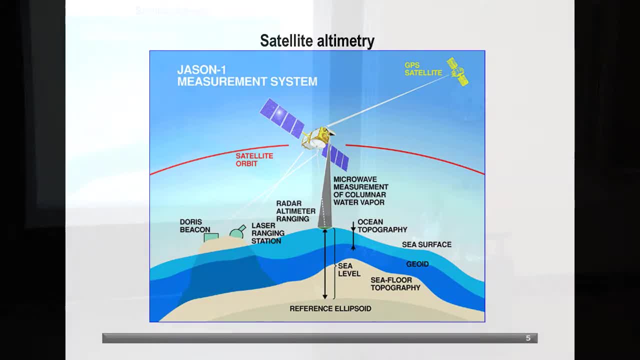 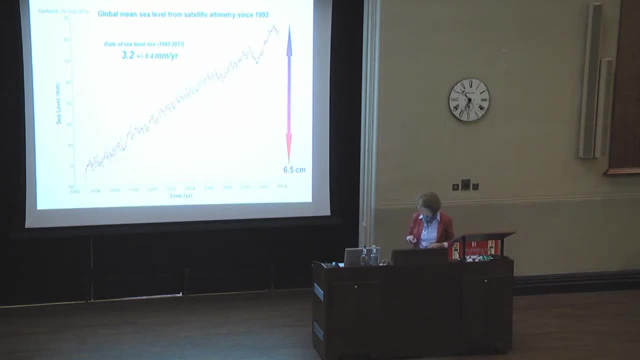 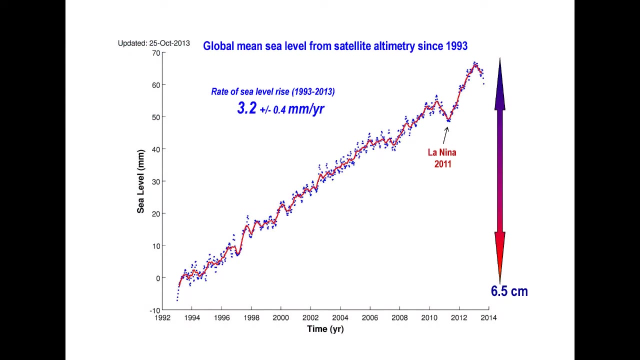 data on absolute C-level. both are important and address different topics, by the way. So here is a recent update of the altimetry-based global mean C-level curve since 1992.. You can see that it's almost linear. 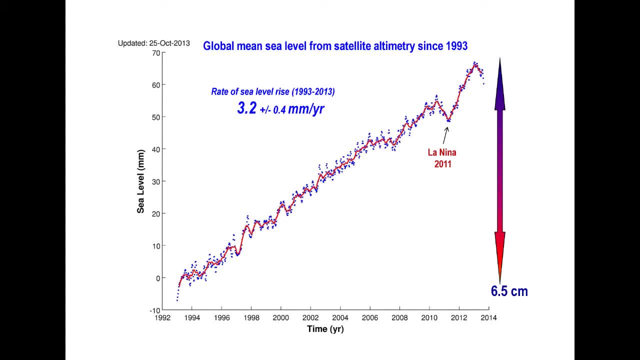 The trend is positive and almost linear, except that I will call about time later some temporary positive or negative anomalies which are related to ENSO events. So the main trend over the last two decades is 3.2 mm per year, with an uncertainty of 0.4.. 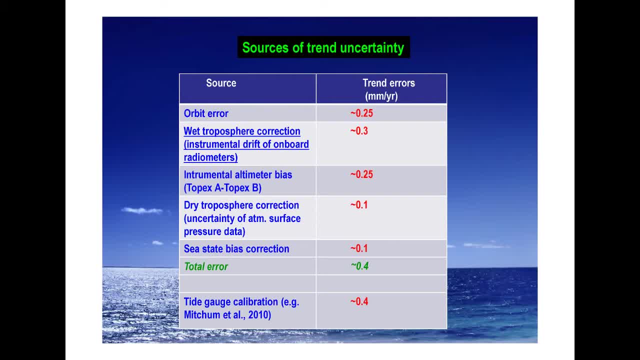 And how is this 0.4 mm per year uncertainty estimated? It's based on various approaches, but I don't know- maybe some other speaker will talk about that. It's based on comparison with state-gauge data, but also on estimates of the various sources of error affecting the altimetry system. 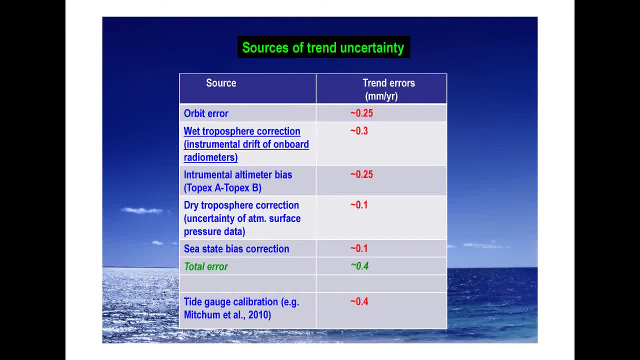 So you can see that the largest sources of error are the orbital error and also instrumental drifts. These instrumental drifts are very important. So you can see that these instrumental drifts are very important. So you can see that these instrumental drifts are very important. 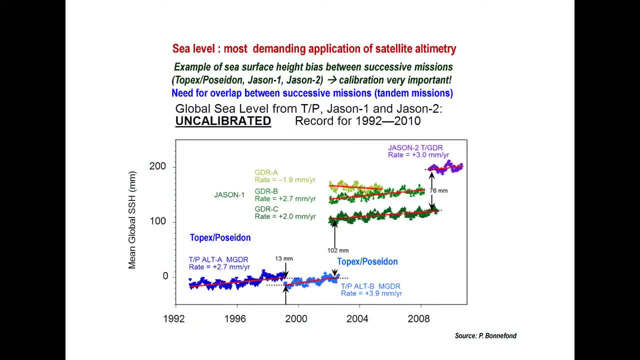 And, as you can see here, on this figure, if you don't estimate the bias between the different missions in the sea surface height measurement as shown here, here you have the sea level from Topex, Topex-A, Topex-B, two instruments on both Topex missions. 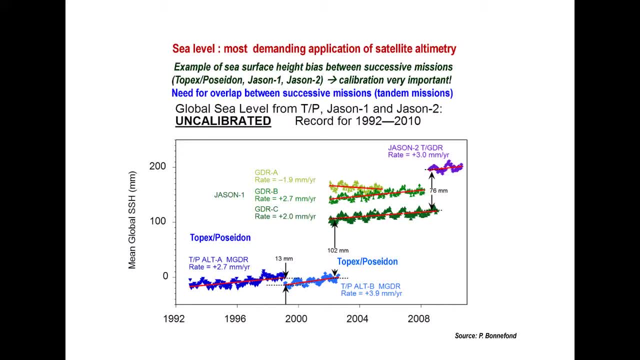 and then Jason-1 and Jason-2, you can see very large bias And it is very important, And it is very important, of course, to correct for this instrumental bias And for that purpose, what is really needed is to have some overlap between the successive missions in order to remove this bias. 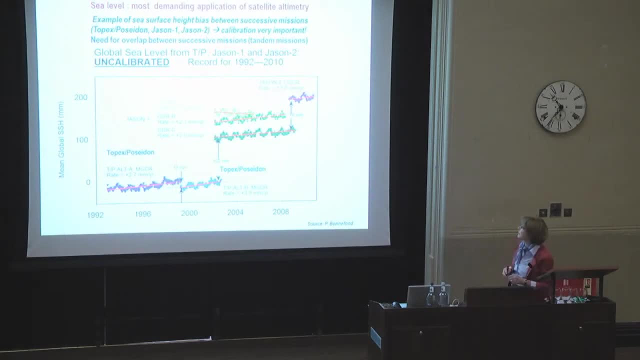 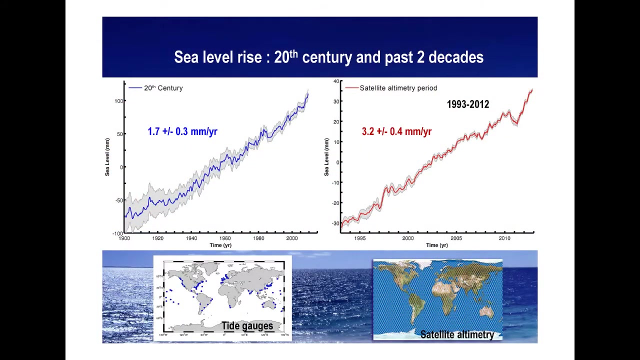 And it is important to recall that the sea level application is certainly the most demanding application of satellite altimetry because, as you know, the signal we try to measure is very low. Okay, Okay, So you have these two curves for the last century: the tide gauge-based sea level curve and the altimetry sea level curve. 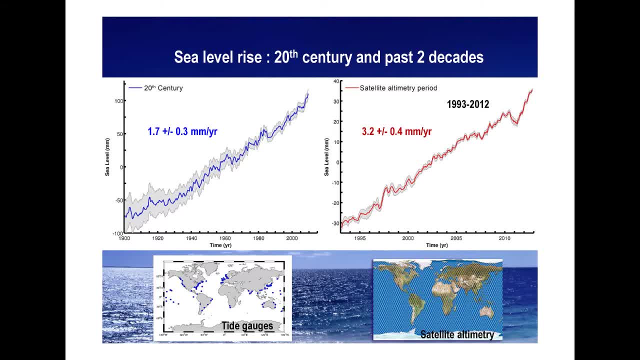 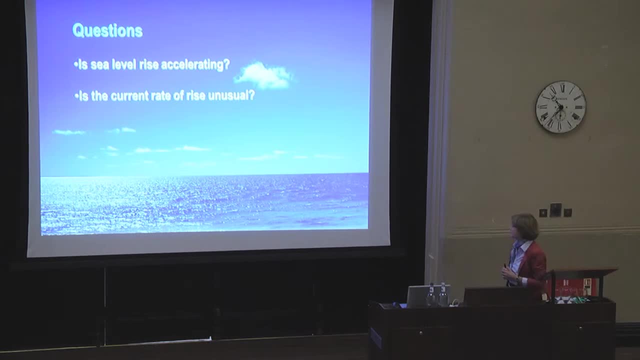 The horizontal scale, of course, is different. The two curves seem to be parallel, but it's not. The rate here is about twice larger than the rate of the last few decades. And one question of course many people ask: is sea level accelerating? 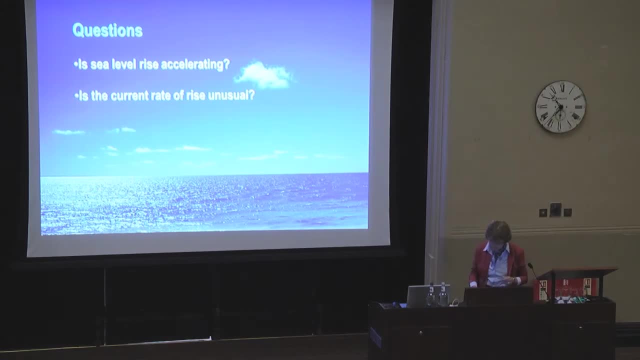 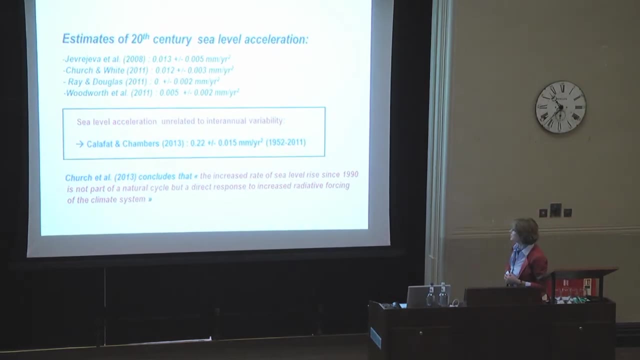 Another question is: is the current rate of sea level rise unusual compared to the last centuries or millennia? So for the first questions, several investigators or groups have tried to estimate an sea level acceleration for the last century, For example. I have mentioned here a number of studies. 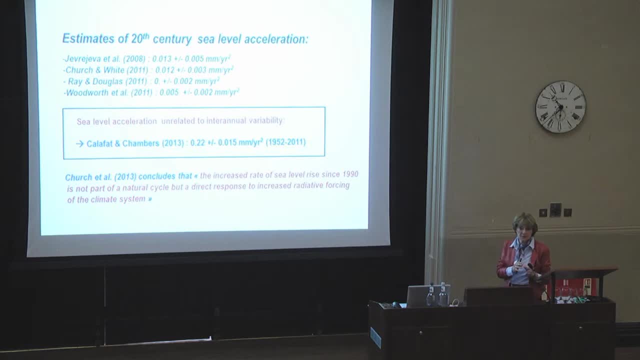 And you can see that the results are different, mostly because the time span considered by these authors are different. A recent paper by Calafat and Chambers provides a new estimate of the acceleration for the last 60 years, which is much larger than the previous estimates. 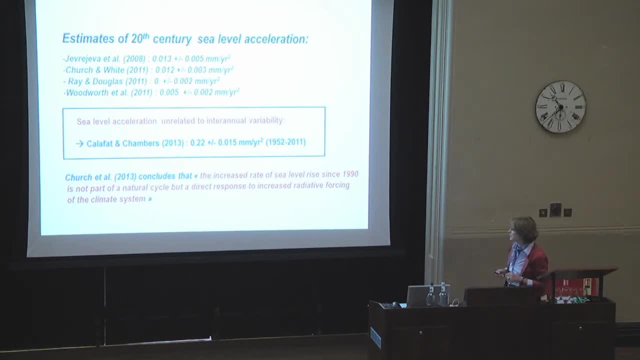 And why is it larger? Because in this study, these authors have tried to remove the internal variation And they come up to a much larger estimate of the acceleration. So their conclusion is that, yes, sea level has accelerated in the last few decades, let's say the last 60 years. 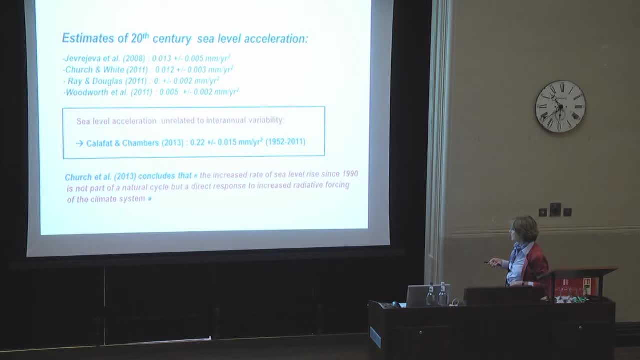 And in another study, Churchill and co-workers, based on comparisons of sea level data with models' output, conclude that the increased rate of sea level rise since the beginning of the 90s is not part of a natural cycle, but it is a direct response of increased radiative forcing of the climate system. 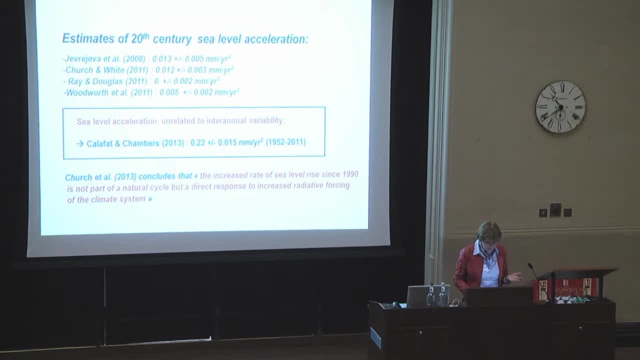 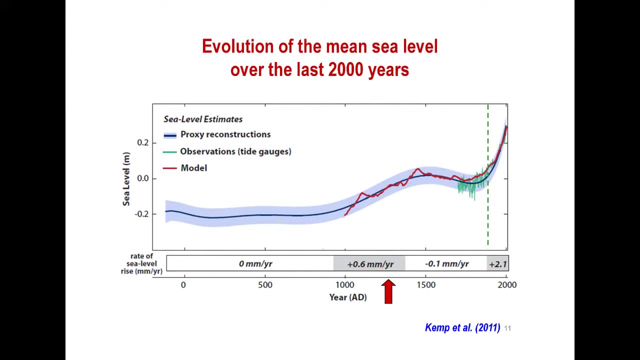 So it seems that really sea level is accelerating and it is not a natural variability signal but it is a response to anthropogenic global warming. So the answer to this question is yes. So the answer to the second question is: is the rate of sea level rise unusual compared to the past centuries and millennia? 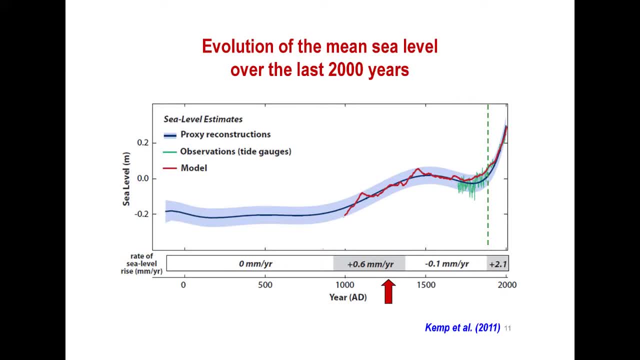 And here also the answer is yes and no. This graph, which is based on a study by Kemp et al, represents the sea level, I will not say global mean, but the best estimate we can have from the sea level variation over the last two millennia. present is here, past is here. 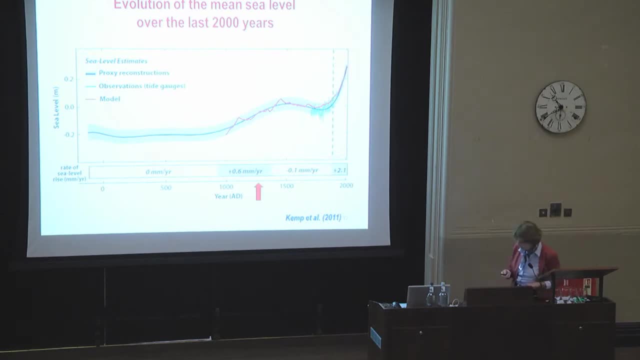 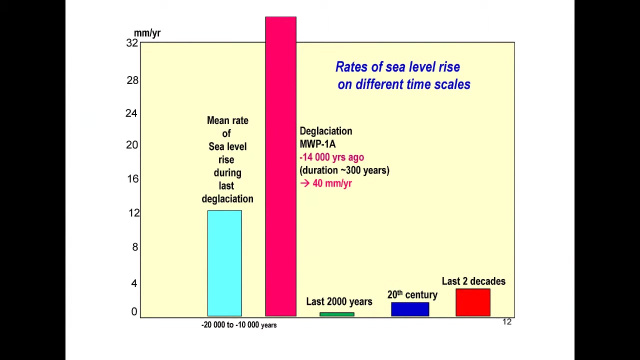 and over this time span, which is based on the salt marsh studies, the rate of sea level rise never exceeded 0.5, 0.6 mm per year until the beginning of the industrial era. So if you compare the last century and last two decades. 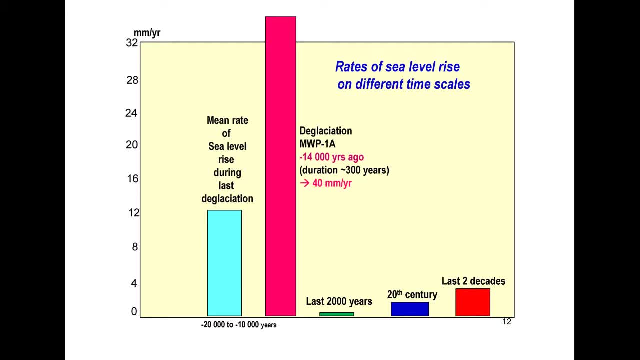 the rate of sea level rise as it is done on this plot. the scale here is the rate to the last 2,000 years' rate of sea level rise. then the answer is yes. The present day rate of sea level rise is unusual. But if you compare now to the mean rate during deglaciation between minus 20,000 and minus 10,000, so the answer is no. On average, the rate during deglaciation was 10 to 12 mm per year. and during some temporary periods it went up to 40 mm per year. Of course, the amount of land ice involved was much greater than it is today, but we can see that a much larger rate can happen in the climate system. So now another question is: 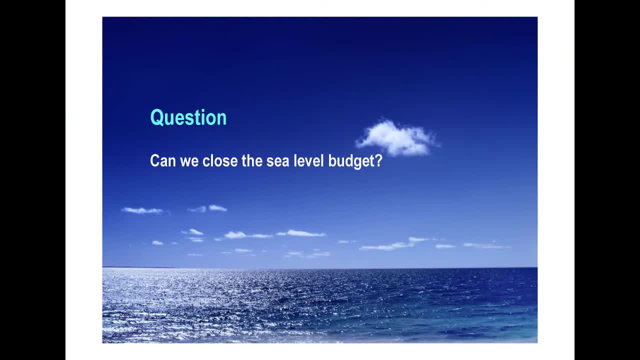 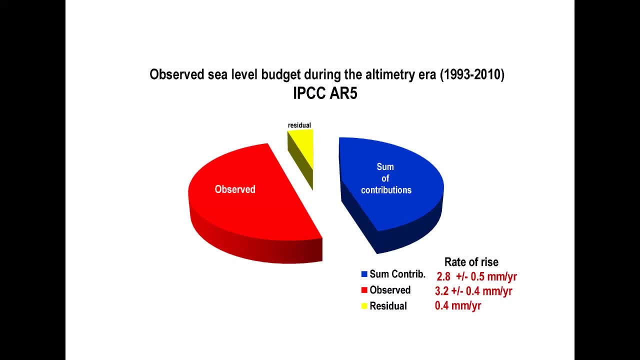 can we close the sea level budget? And the answer is yes, And this is the result shown in the IPCC year 4, with the observed rate of sea level rise. So I will talk only of the altimeter era. I think Jonathan will talk about the whole century. 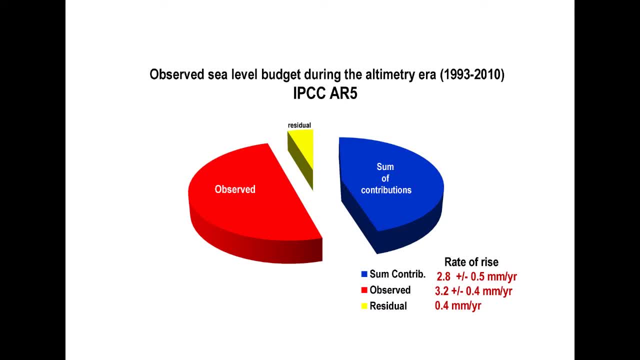 So I just talk now about the last two decades, almost the last two decades. So here we have the observed rate of rise of 3.2 mm per year, and here is the sum of the contribution as estimated using data observations. 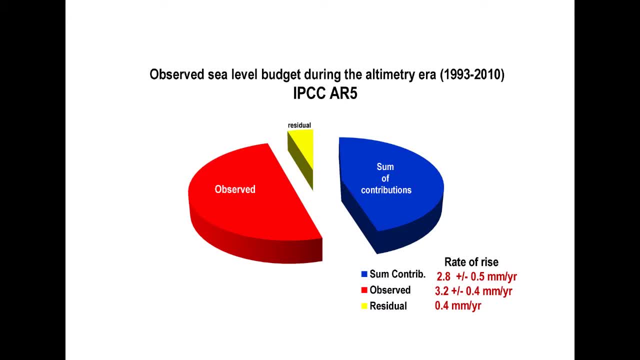 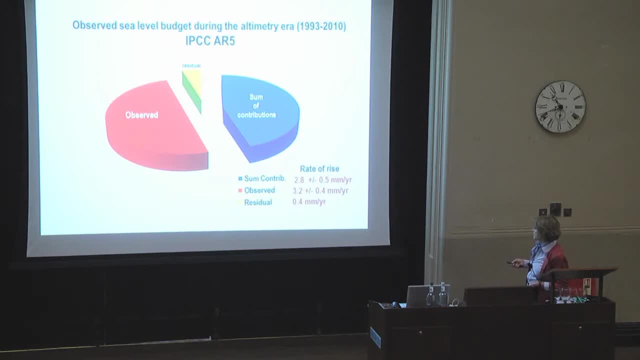 We will go in more detail in a moment. So you can see that we can almost explain the rate of sea level rise observed by satellite altimetry. So there is a small unexplained residual, but which is not very large. So now what are the details? 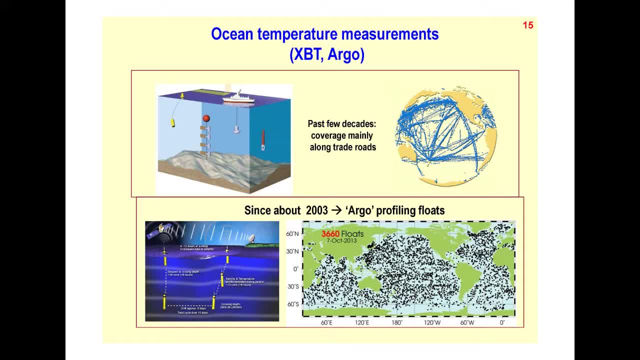 Concerning the thermal expansion contribution, you know, I don't recall, but I think the audience here is very familiar with sea level and contributions. So there are two contributions: thermal expansion in terms of global wind and land ice melt. So the thermal expansion contribution. 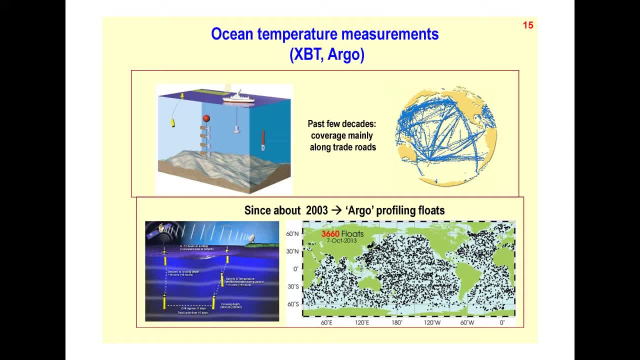 the thermal expansion contribution is estimated for the last few decades using XBT data measured from ships and, since about 10 years, from the Argo profiling floats with global coverage, as you can see here. And here is another plot from the IPCC AR4,. 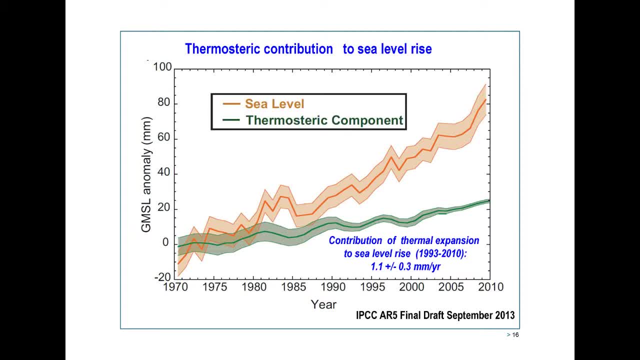 AR5, sorry that shows since 1970, the sea level curve, global sea level curve and the thermal expansion contribution On the other over the period 1993 to 2010,. more or less the altimetry era. 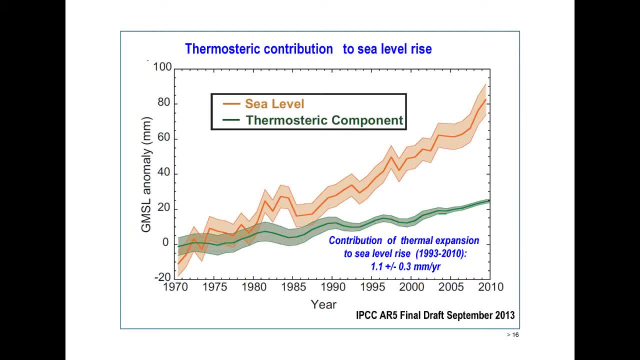 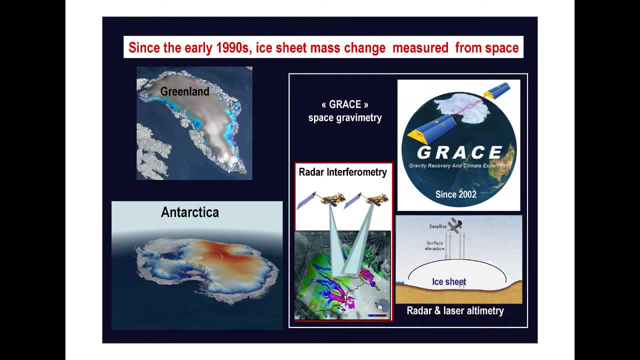 the estimate is 1.1 mm per year, which is about 30%, a little more than 30%, around 30%. sorry So I will not go into the detail about land ice, because Jonathan Bamber, I think. 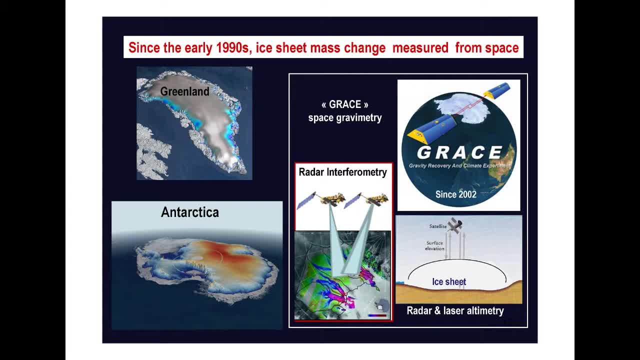 will talk about that, but I just want to show the results. As you know, the mass balance of the ice sheets are measured using space techniques since two decades. Just to recall the techniques: altimetry, laser and radar altimetry. 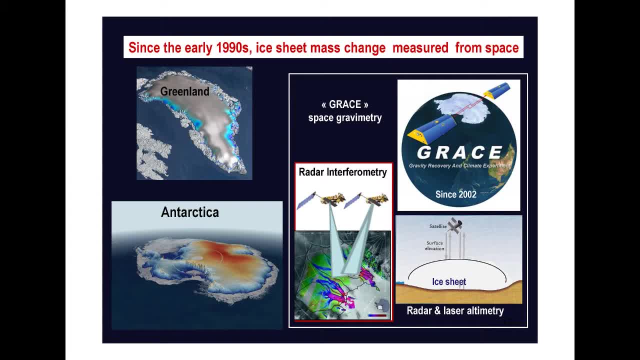 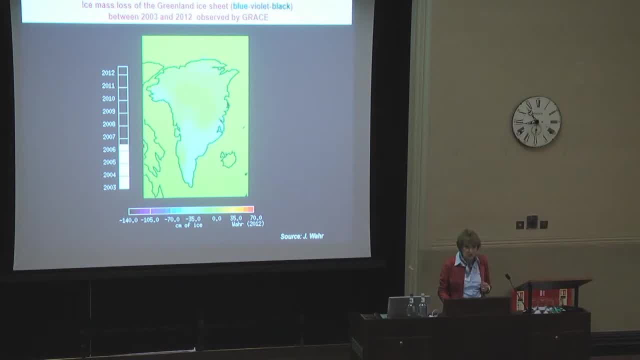 radar interferometry in SAR and gray space gravimetry. Just I want to show you a result from GRACE. This is an animation provided to me by John Waugh from the University of Colorado, and it shows the loss of ice mass. 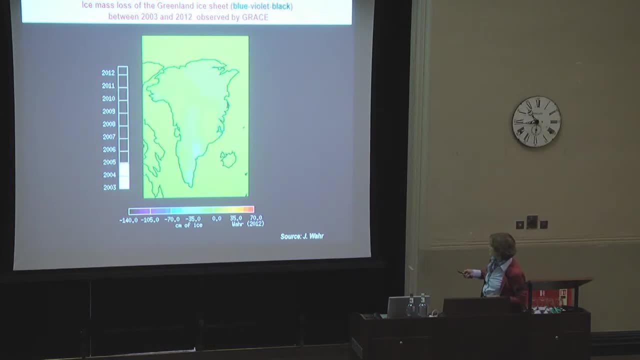 for Greenland since 2003.. So it started in the south, south-east coast of Greenland and then propagated along the western coast. I am sure you will talk in more detail about that. Okay, So just to show you a curve, a figure. 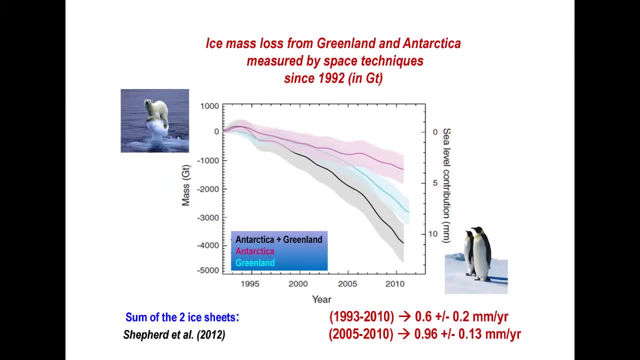 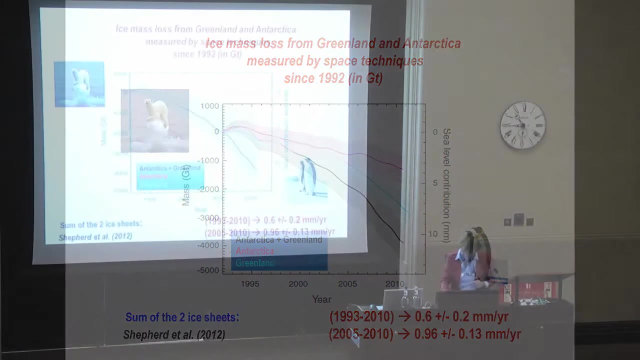 which is from a recent publication, almost one year now, from Shepard and co-workers, trying to reconcile results from different groups and from the different techniques. we have here the decrease in mass, of Antarctica, Greenland and both ice sheets. Now I will not talk about the glaciers. 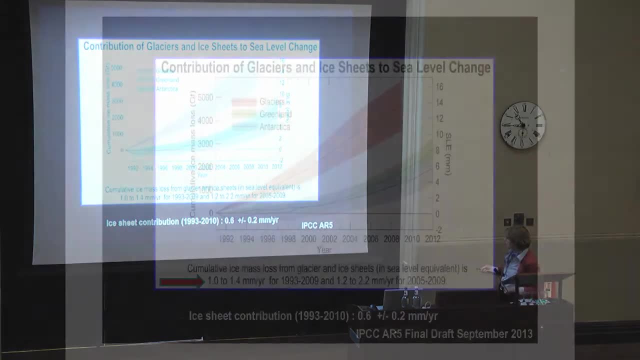 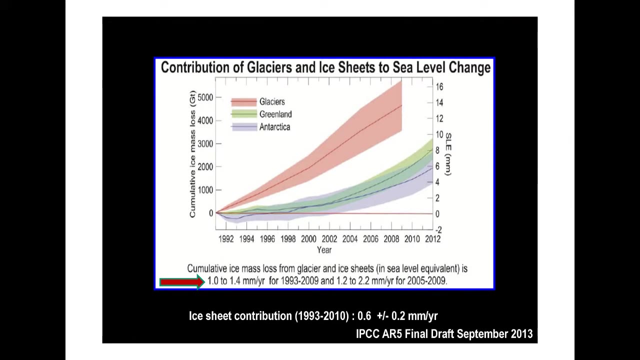 And here just a summary of the land ice contribution And again, this is a figure from the IPCC-F5.. We have, so it is presented differently. So we have the ice sheet contribution here and the glaciers contribution, And on average, 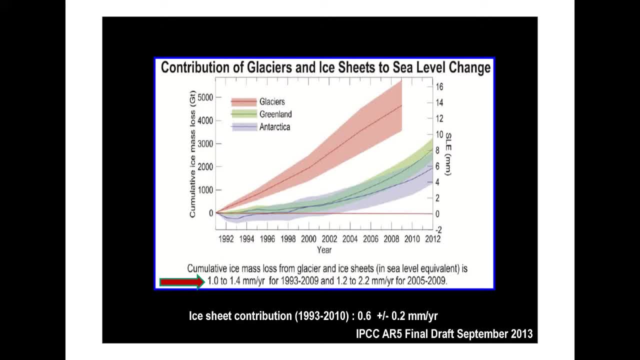 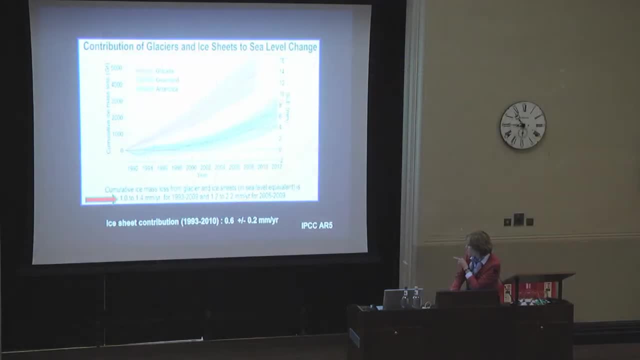 over the period 1993 to 2000,. 2010,, which is the period considered by the IPCC-AR5,, the land ice contribution is on the order of 0.6 mm per year. And no, sorry, this is just the ice sheet contribution. 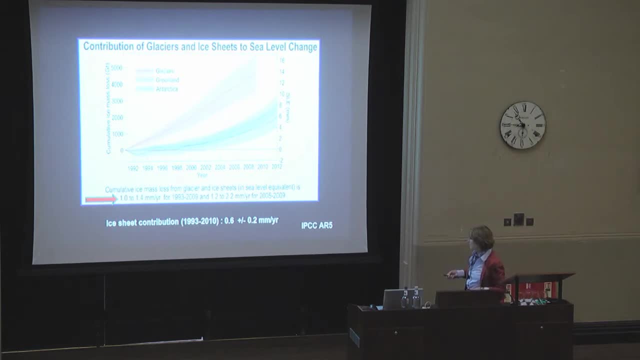 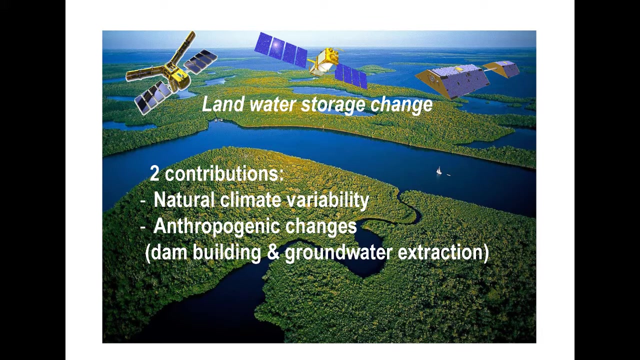 And the total land ice, glaciers and ice sheets is between 1 and 1.4 mm per year for the altimetry era, with some acceleration in the recent years. So now there is another contribution, which is land water storage change. 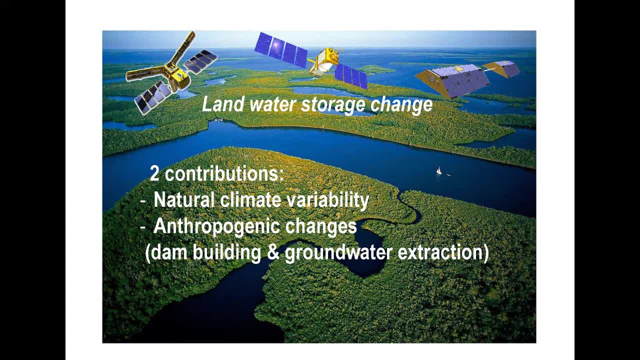 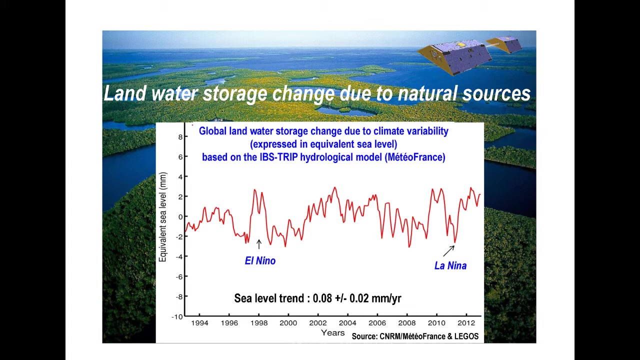 Land water storage can contribute to sea level. There are two sources of contribution. One is natural climate variability And the other is anthropogenic change due to dam building and groundwater extraction. So here we have a plot that shows the natural variability component. 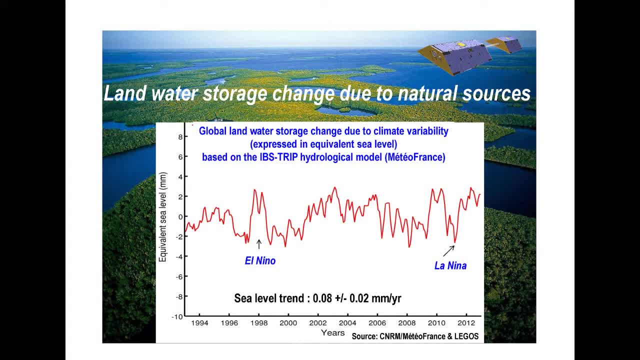 This is based on. Sorry, there is an error here, It's ISBA. This is based on the hydrological model developed by Meteo France in France, And it shows the land water contribution due to natural climate variability expressed in sea level equivalent here. 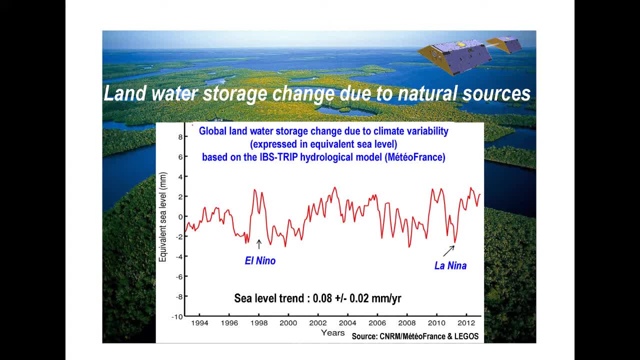 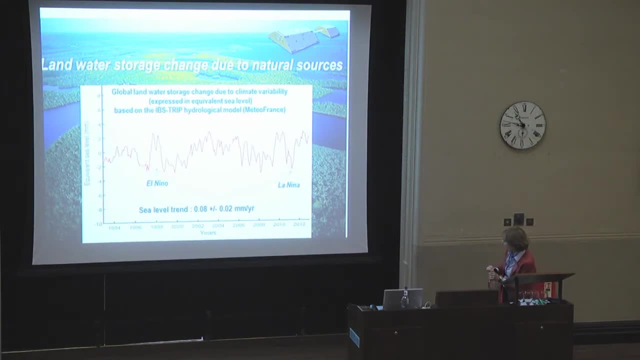 And what you can see is that there is no long-term trend. This was known before by previous studies. There is no long-term trend. The trend over the last two decades here is 0.08 mm per year, As you know, since 2002 or 2003,. 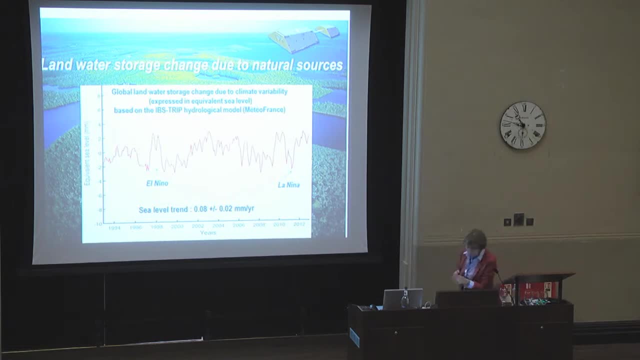 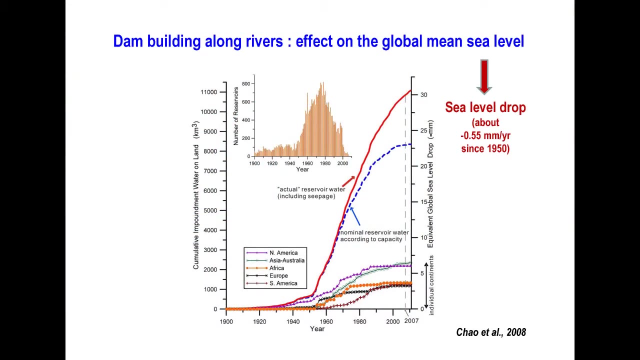 we can estimate this component using GRACE, But prior to GRACE we have to use models. Now about the anthropogenic. These two contributions- dam building and groundwater extraction- are relatively large contributions but of opposite sign And this contribution remains very uncertain. 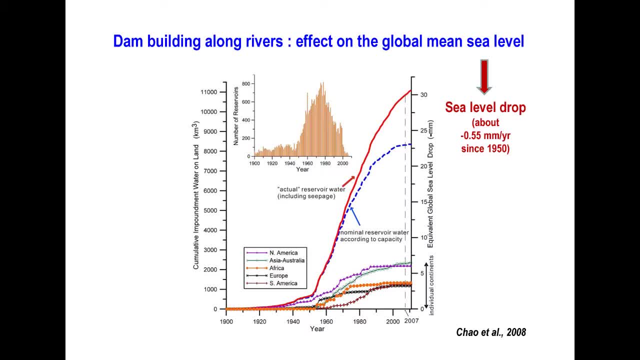 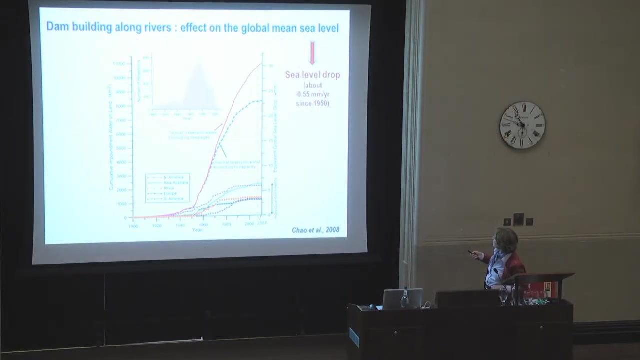 Here is a plot from Chao et al 2008 that shows the cumulative water volume improvement behind dams for the last century, And this author estimates that dam building led to sea level drop of about minus 0.55 mm per year since 1950.. 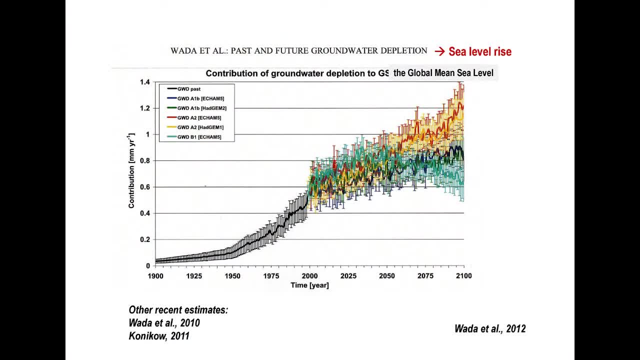 This is the other contribution due to groundwater depletion. Sorry, This is based on. this is a figure from WADA and co-workers, a paper published last year, But there are also other studies. I have no time to go into the detail. 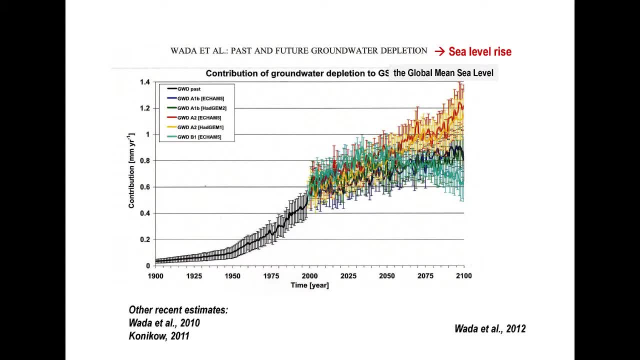 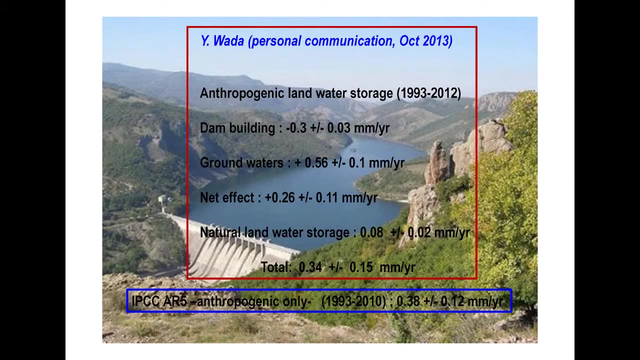 And here this is based on observation And you have projection, but I will not talk, of course, of projection. I think Jonathan Gregoire will talk about that. So if we, the order of magnitude of this effect for the last two decades are the following: 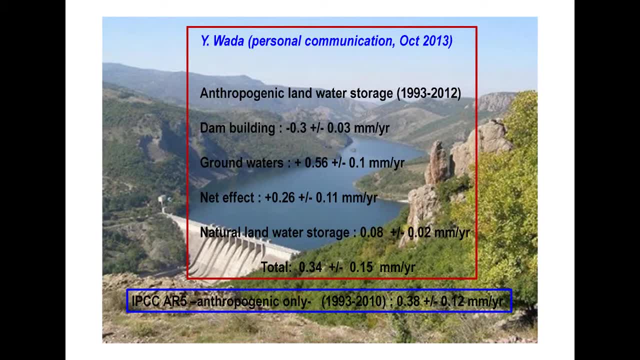 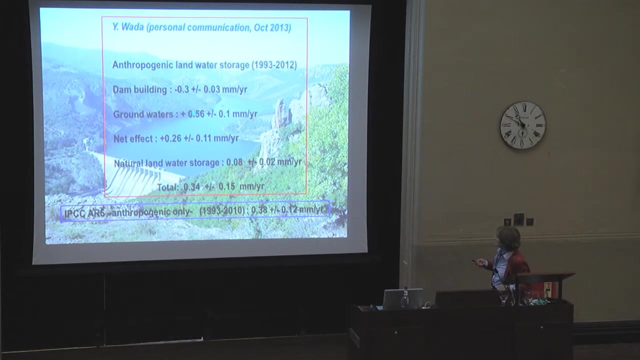 This is the numbers from that I got from WADA directly for the period 1983 to 2012.. So the dam building contributed negatively to sea level by minus 0.3.. The groundwater depletion or extraction contribute positively to plus 0.56. 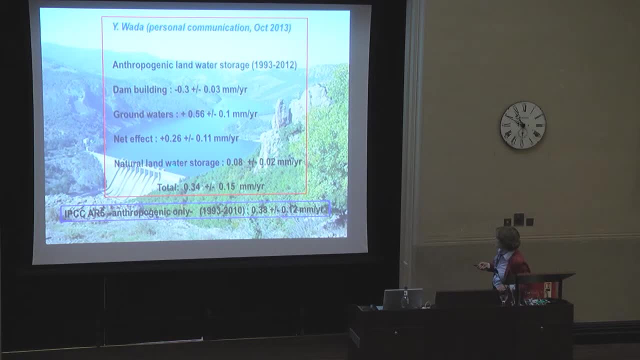 and the net effect is 0.26.. So if we add now the natural contribution, we come up with the value of 0.35, which is very big compared to, for example, Antarctica or Greenland. So in the IPCCR4,, 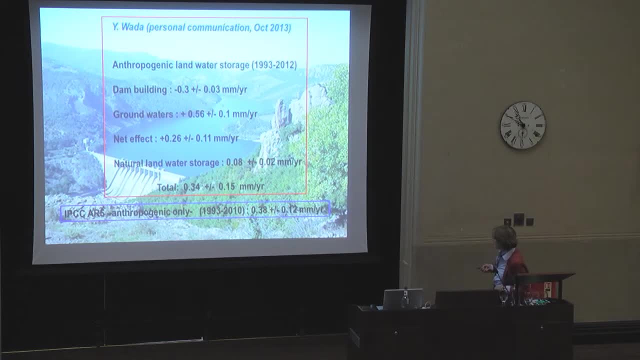 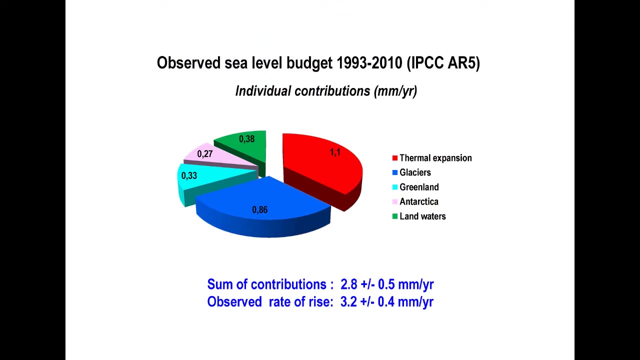 for this period, which is not exactly the same, the number used was 0.38.. Okay, so now we have the individual contribution. You can see the relative importance of each contribution: thermal expansion glaciers, which are the largest contribution, and the other contribution. 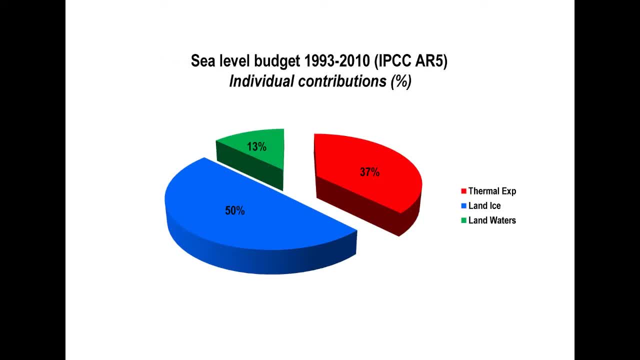 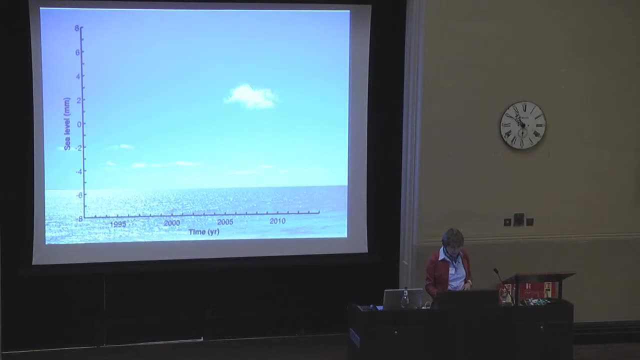 And here a similar plot shown differently: Land ice, which is by far the largest contribution, followed by thermal expansion. Okay, so, this was the IPCCR4 results about sea level observations. Now I would like to talk a little about the inter-annual variability. 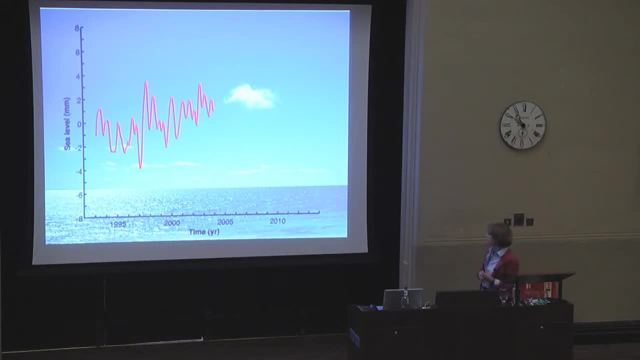 If we remove the linear trend from the global mean sea level curve estimated by satellite altimetry, we come up with a curve like this which shows: oops, I'm sorry it's gone, maybe I don't know if I can show it again. 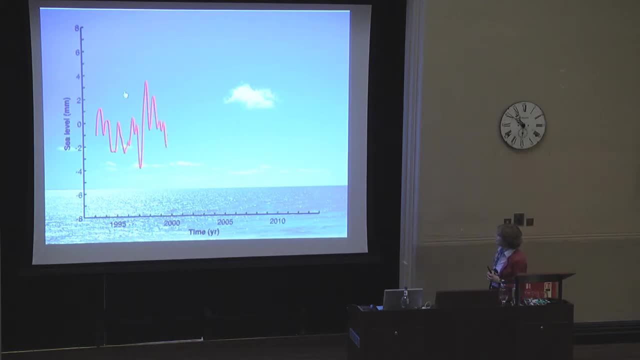 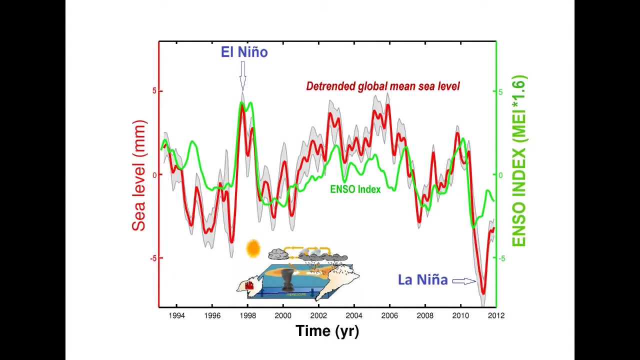 Large inter-annual anomalies on the order of several millimeters, which is huge, And, as shown by a number of studies in the recent years, this inter-annual fluctuation in the global mean sea level are strongly related to El Niño. El Niño-La Niña. 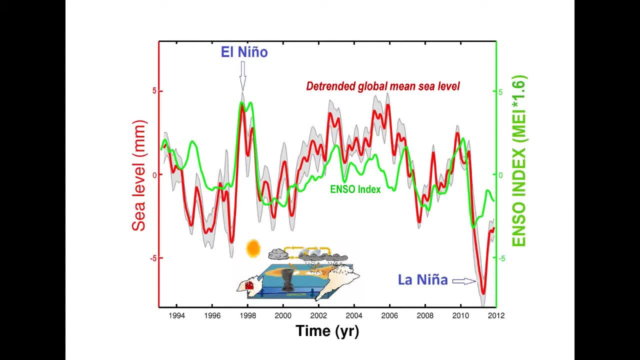 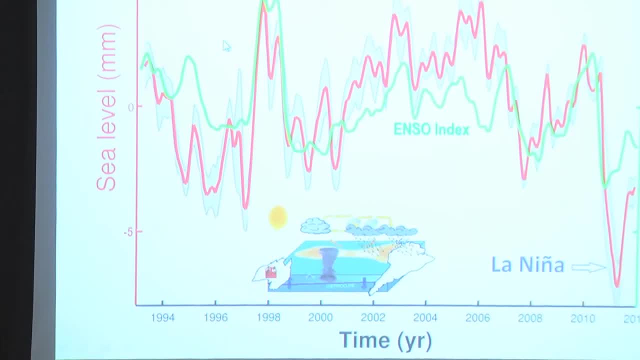 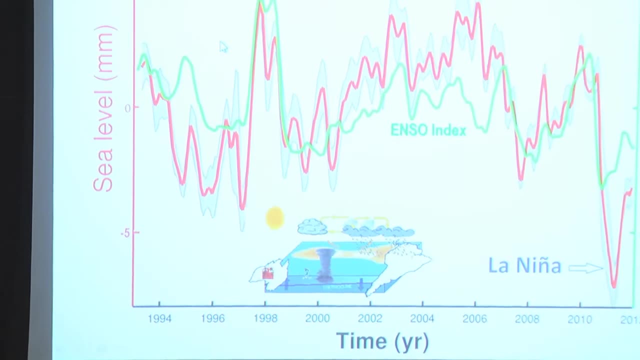 that is the ENZO index as shown on this figure. Here again, the red curve represents the detranode global mean sea level over the altimetry era And the green curve here represents an ENZO index. here the MEI. 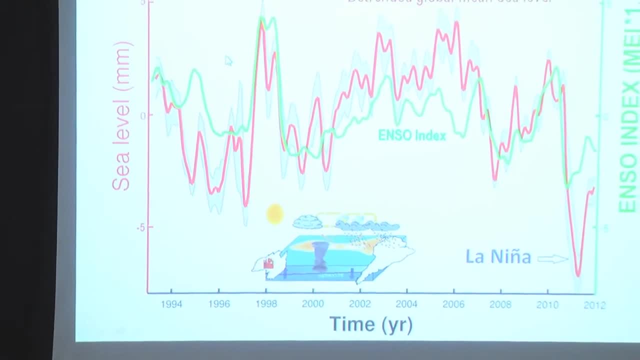 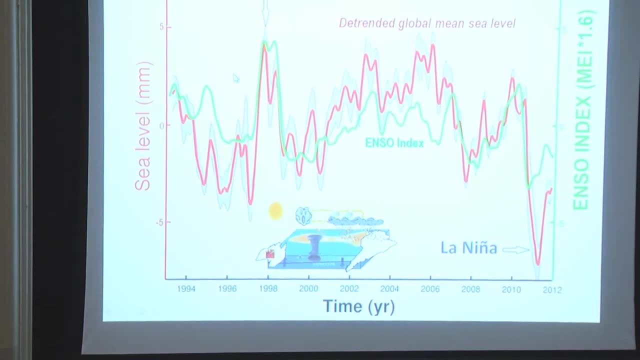 And what you can see here. what you can see is that when you have an El Niño here, for example, there is a positive anomaly in the global mean sea level, and when there is an La Niña, there is a negative anomaly. 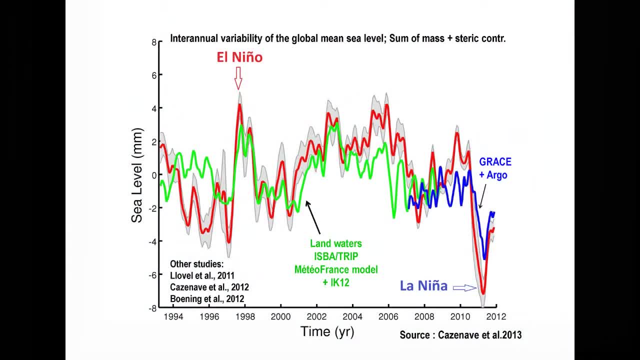 So several studies in the recent years have tried to understand the cause of this, of this positive and negative anomaly, and how they relate to ENZO events, And these studies have shown that it is mostly mainly a mass effect which is responsible for this anomaly. 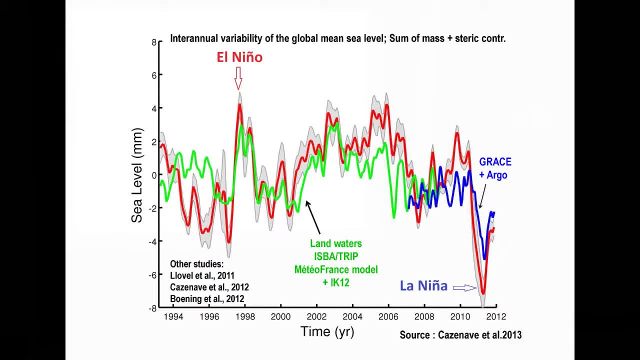 Typically when there is an El Niño, there is more rain over the tropical ocean, mostly the tropical Pacific, and less rain over river basin in the tropics. So this causes a positive anomaly of the global mean sea level And we have the opposite. 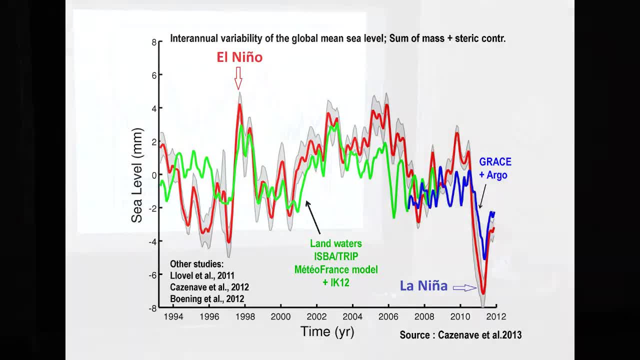 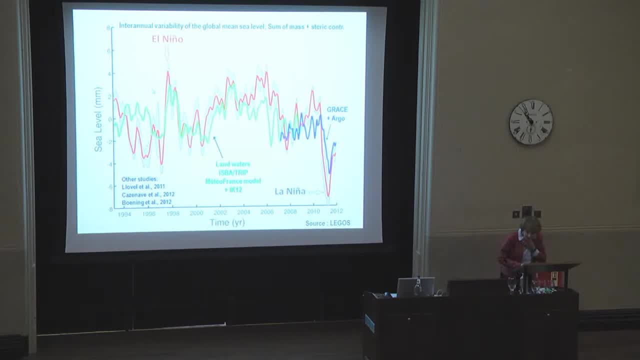 during La Niña, And here you can see a quantitative comparison. I'm sorry, I have a, I was sick during the weekend, so Here you can see a quantitative comparison between the detrended global mean sea level, which is a red curve again. 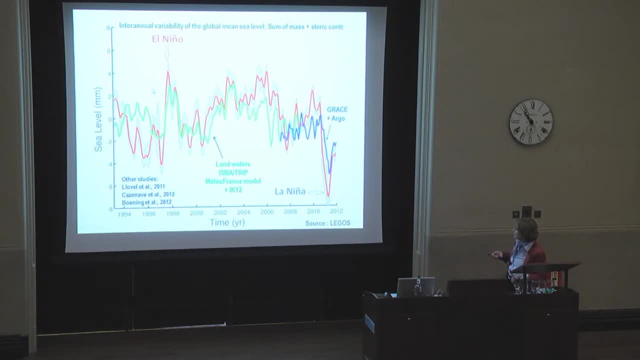 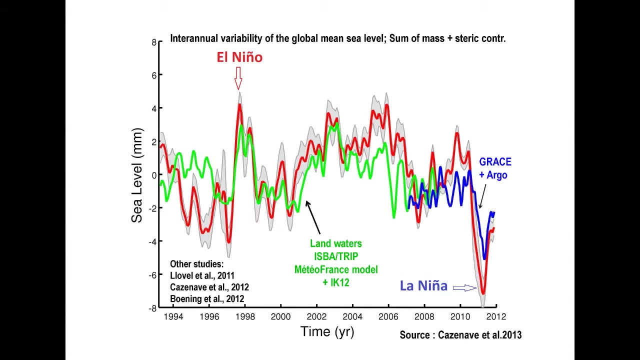 and an estimate of the land water contribution, here again based on the Meteor France model up to 2008.. And in blue, here based on GRACE, because, as you know, GRACE can estimate the land water contribution On this plot. 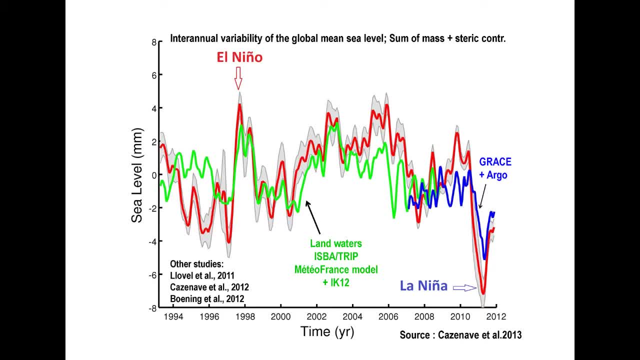 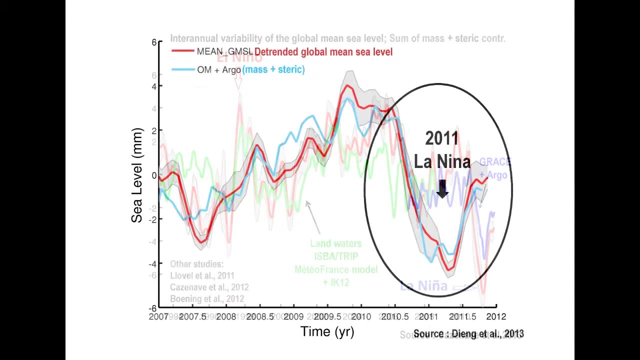 a small contribution from the inter-neural steric effect. thermal expansion effect has been added because there is a small contribution from thermal expansion but the main effect here is a mass effect. If we focus on the recent La Niña, you know that. 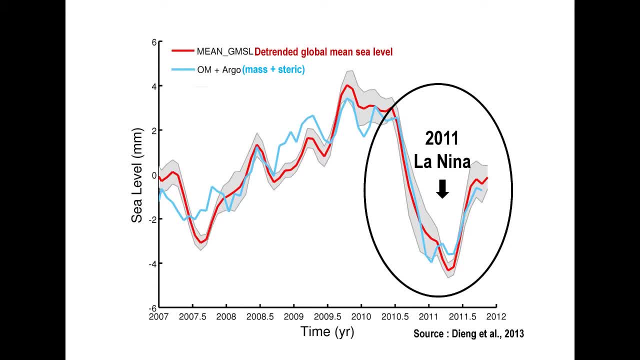 in 2010, the global mean sea level curve dropped by more than 2 mm- nearly 4 mm, by the way- And some climate skeptic claims that sea level is no more rising, it's falling, But it was just a temporary effect. 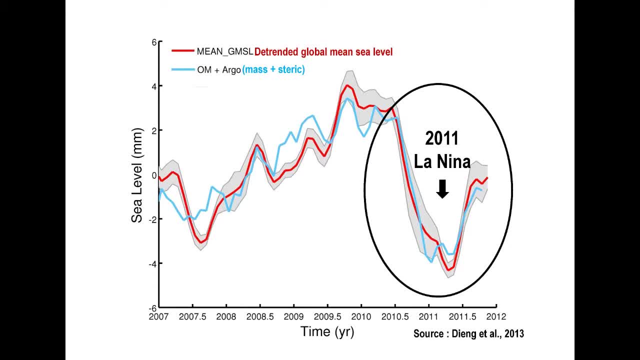 due to the strong La Niña that occurred in 2011.. And here in blue you have the curve which represents the mass plus the small steric contribution to this La Niña effect. The main effect here is a mass effect again. 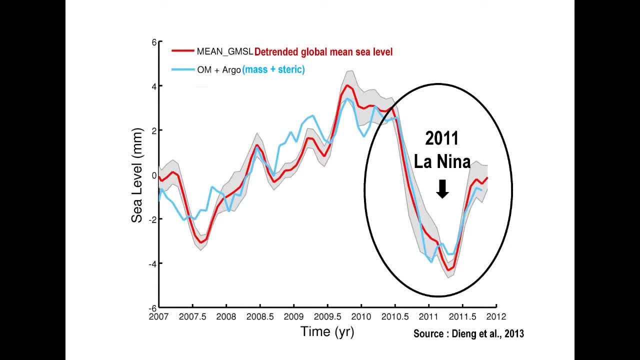 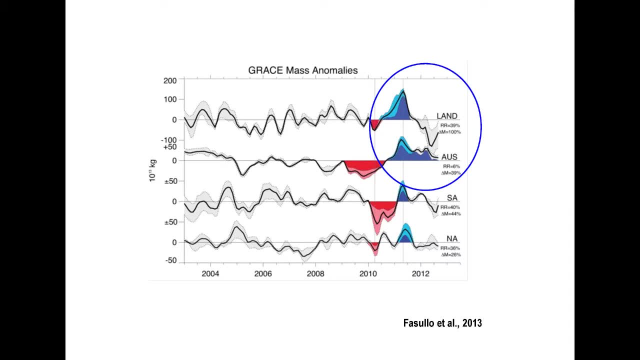 with less rain over the ocean and more rain, which means more water in the river basins on land. In a recent study published during summer by Fasulo and co-workers, the author showed that the main contribution to the land water the main region contributing. 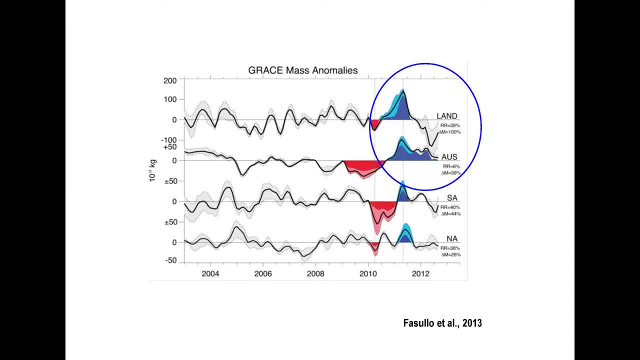 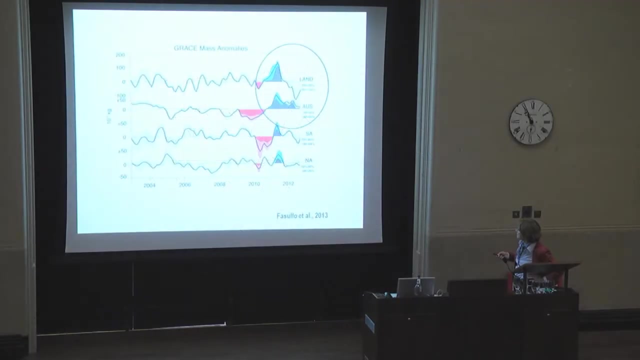 to the positive land water effect was Australia. Here on this curve, you have the mass anomaly, land water storage anomaly, based on gross observations since 2003.. And you have this big positive anomaly during the La Niña, 2011. La Niña. 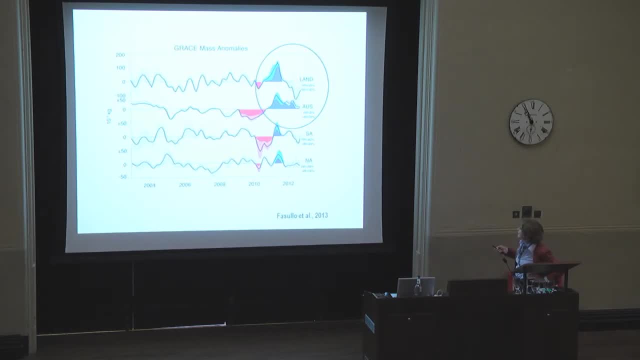 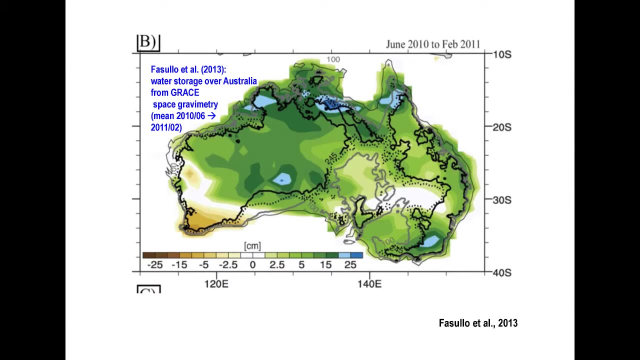 And here you have the contribution from different regions And you can see that the largest contribution comes from Australia. And this figure, again from the same study, shows the very strong positive land water storage in Australia over Australia during this La Niña effect. 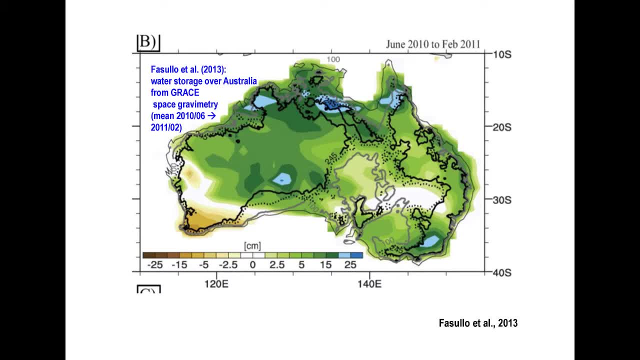 So, in particular, you can see large positive anomaly here here. Much water, by the way, all over the region, And this author explained this by a particular condition due to the Indian Ocean dipole and the southern. how do you say? 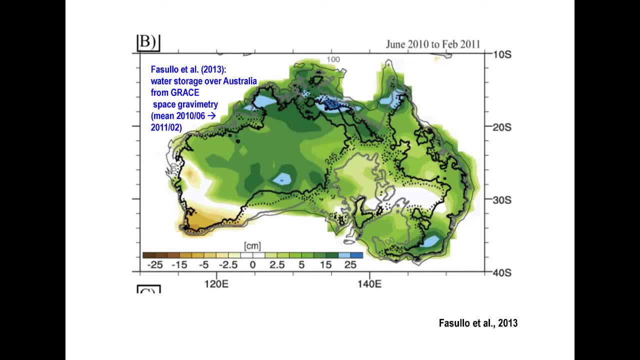 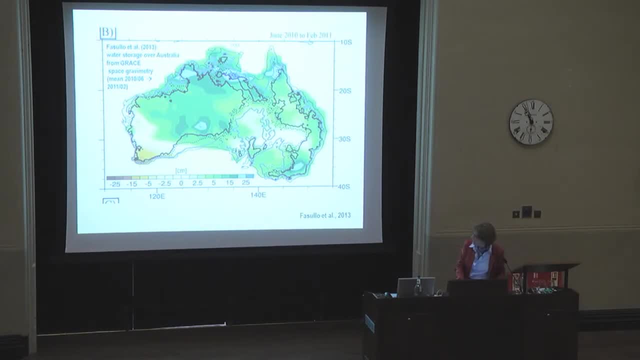 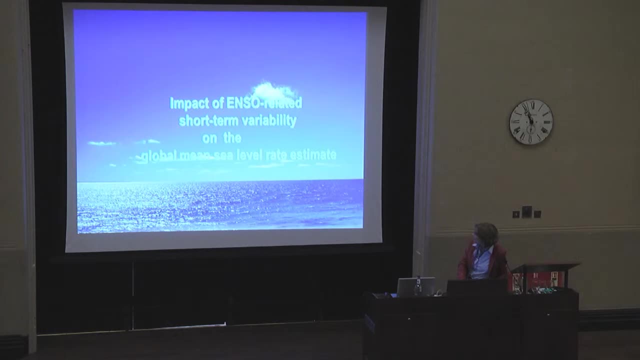 southern anomaly mode, I don't remember, Okay Anyway- particular meteorological condition during in the southern ocean, the southern hemisphere, during this La Niña event. But I would like to show some results which are under. we are working on this problem. 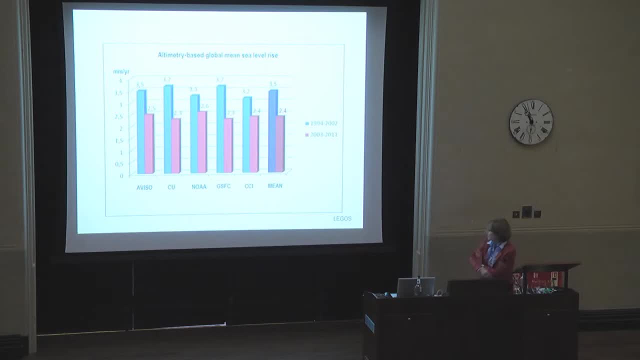 in our group. If we remove, if we compare, the mean weight of sea level rise during the first decade of the altimetry era- these are the blue bars here. using data from different groups, processing the altimetry data, we find that 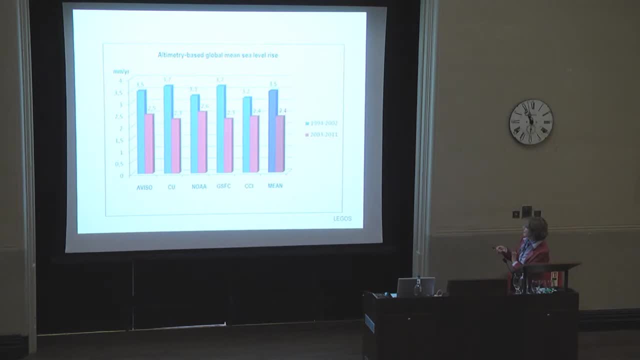 for the first decade of the altimetry era, the rate of sea level rise was on the order of 3.5, something like that: between 3.3 and 3.7 mm per year, with an average of 3.5.. But during the following decades- that is, the last decade- the rate was seems to be much lower, by about 30%, And it was suspected that this was due to this succession of La Niña effect, which provided negative anomalies in the global mean sea level. 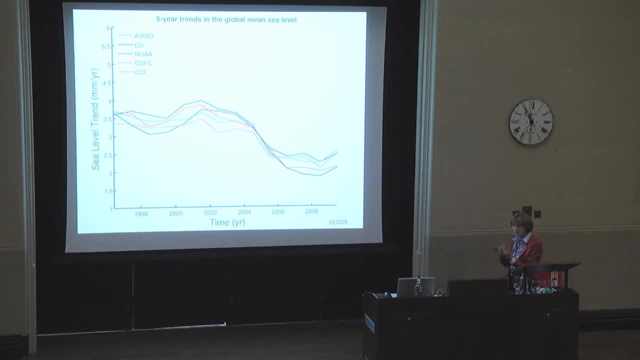 And if we correct for that, maybe the rate will be different from what we observe Here. so here it's, before doing this correction, what is shown here again for all. altimetry data sets five-year trends of the global mean sea level. 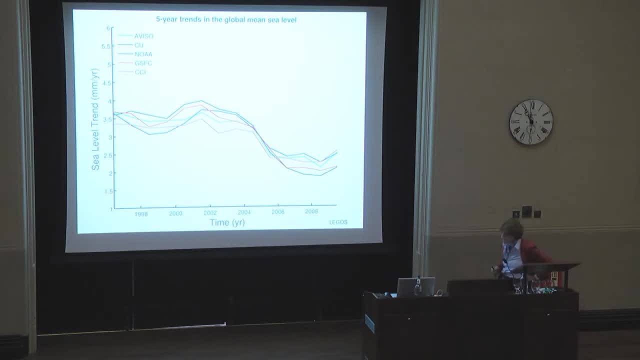 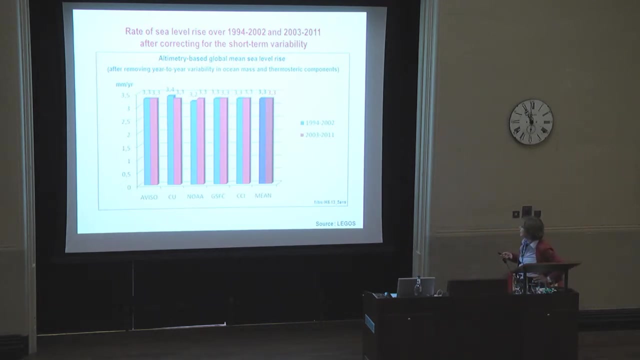 and you can see this decrease, this drop during the last decades. Now, if we remove quantitatively this mass effect, we find that for the last decade the rate of sea level rise is, on average, exactly similar to the rate of the first decade. 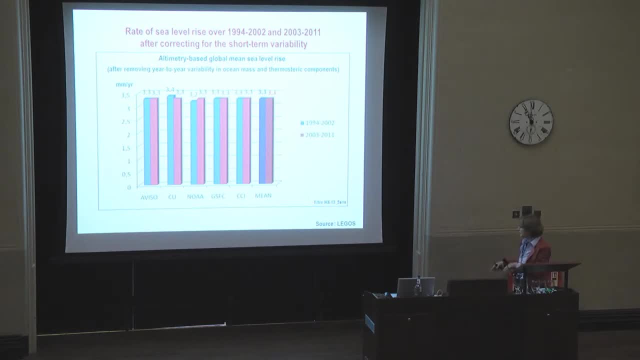 So the result is that the apparent decrease during the last decade is mostly due to interannual variability related to La Niña events- ENSO events, but mostly La Niña- And this result seems to indicate that sea level is continuing to rise with a constant rate. 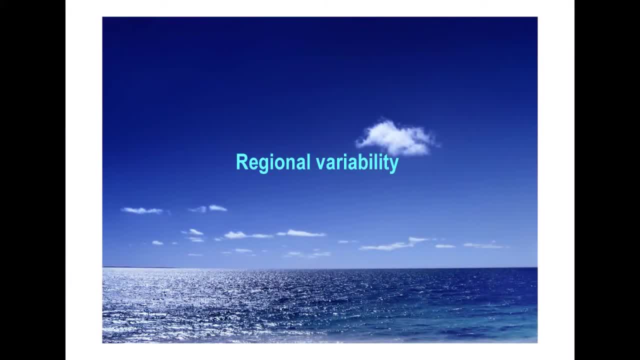 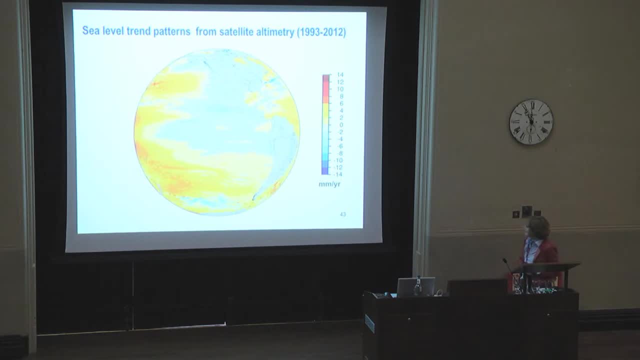 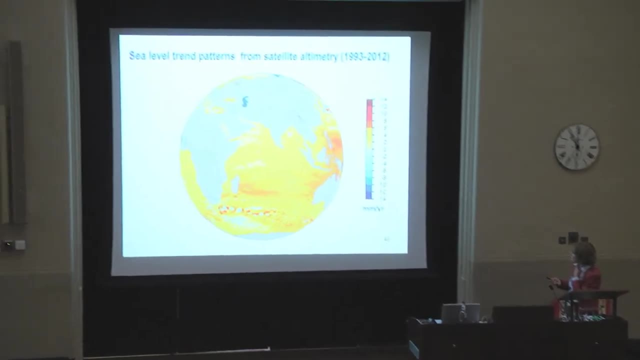 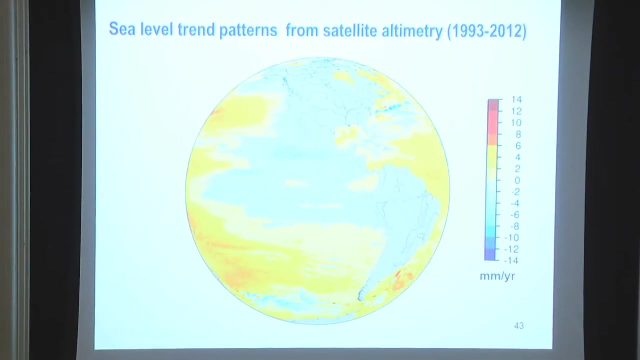 Okay, now I move to the last part of this presentation. It's about the regional variability. This is one known figure that shows- sorry, the sea level trend patterns measured, observed by satellite, I'm sorry, satellite altimetry during the altimetry period. 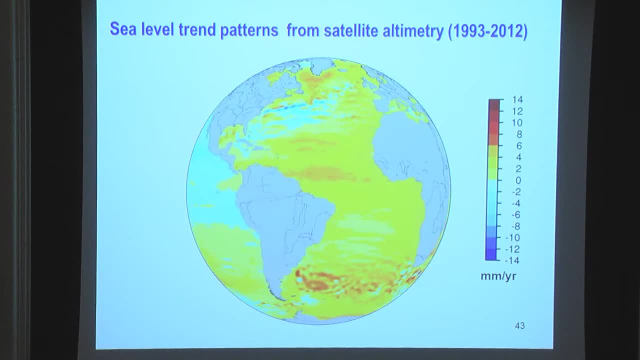 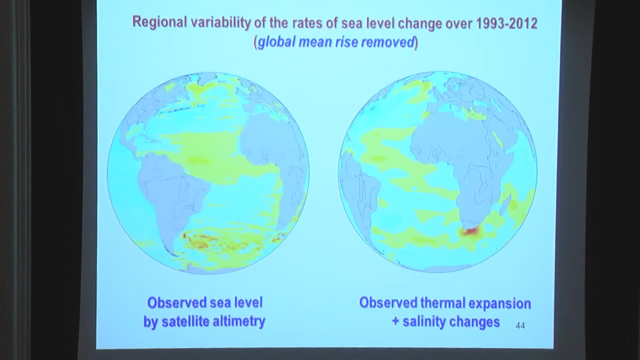 With the with larger threat of rise in, as you know, in the Western Tropical Pacific, North Pacific, North Atlantic and so on. So it is now well known that this, this special trend patterns, are due to non-uniform thermal expansion. 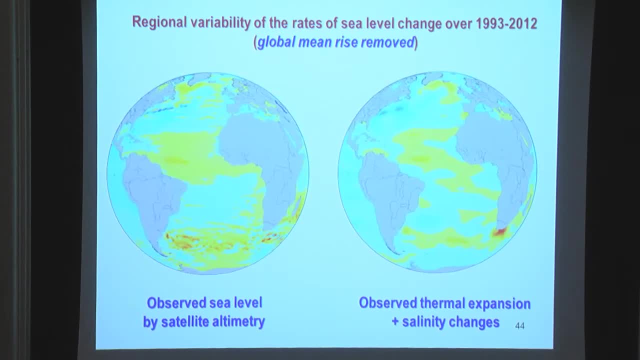 Normally okay. So on the left it is exactly the same figure as the previous one, except that here the global mean rise has been removed. And on the right you have the special pattern in thermal expansion, Again with the global mean. 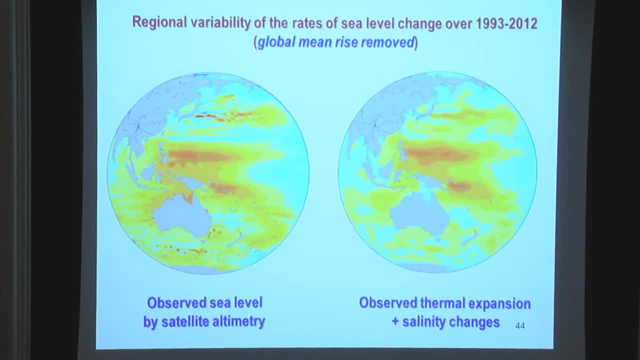 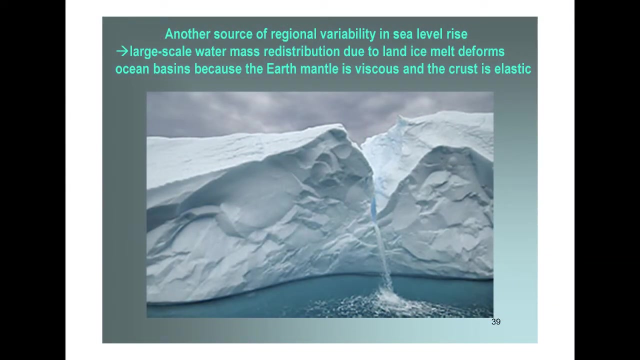 rise removed And you can see the very good correlation between the two. So this is known for several years now. One question is that if we remove this thermal expansion contribution, can we detect other source of regional variability? We all know that there are other source. 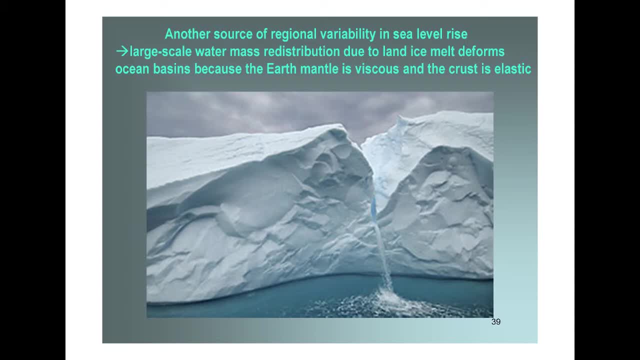 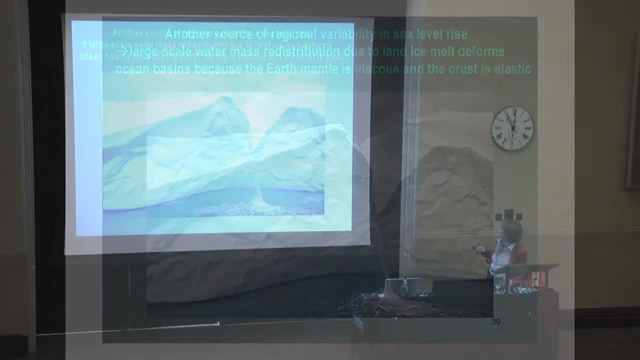 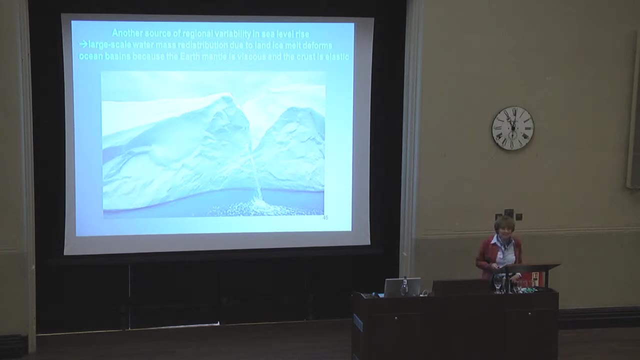 of regional variability, In particular the, the process linked to the solid earth response to large scale mass redistribution associated with past and present land ice melt. Mark is working on that. I know that there will be a talk tomorrow by Giorgio Spada. 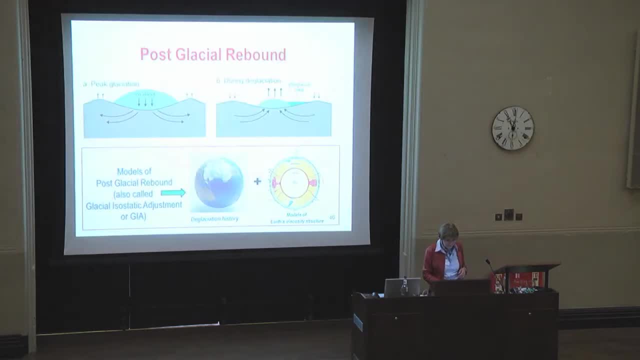 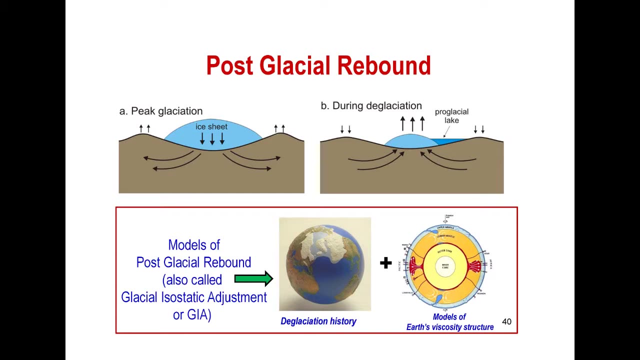 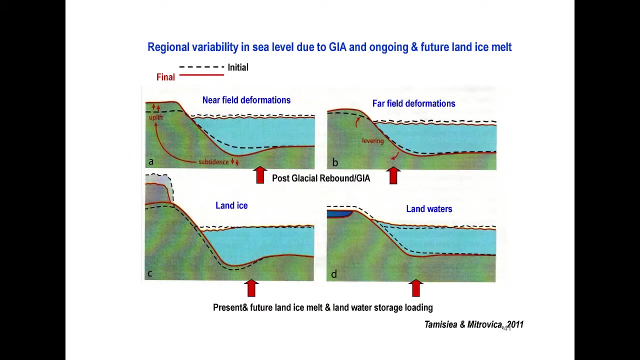 on that topic. So this is the well known phenomenon of post-glacial rebound. I will not go into the detail of this And these two fm, that is, post-glacial rebound and present there and also future land ice melt. this is an 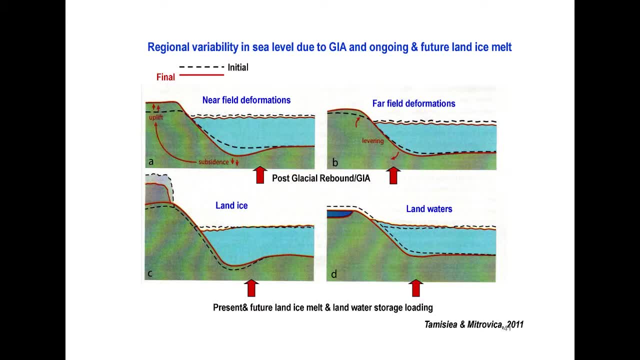 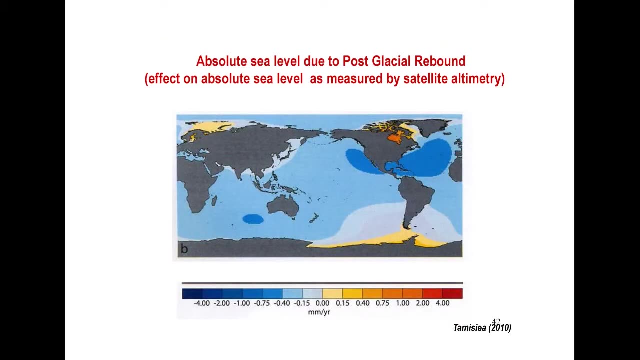 example of post-glacial rebound that is present in the sea level. And this is the example of post-glacial rebound on absolute sea level as measured by satellite limit weight. So the non-regional variability can reach in some region, I mean. 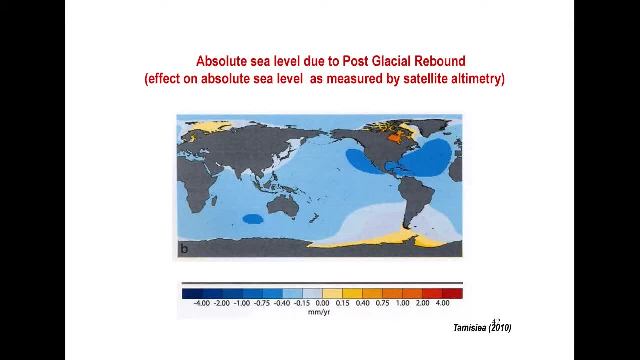 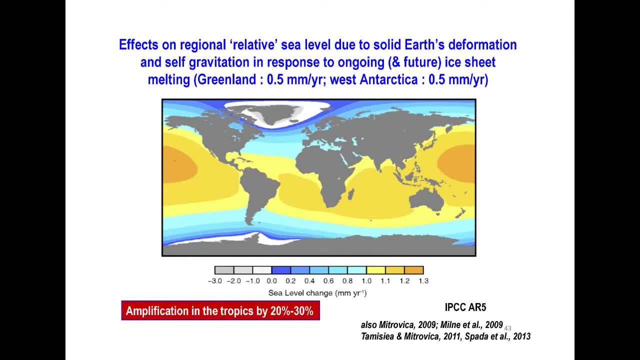 here over the ocean, minus 0.4.. And here is. this is a map from the IPCC R5 that shows the effect of present day Greenland and melting weight in terms of sea level equivalent of 0.5 mm per year for Greenland, and 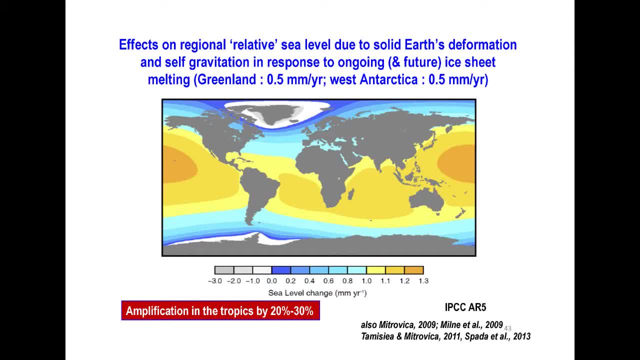 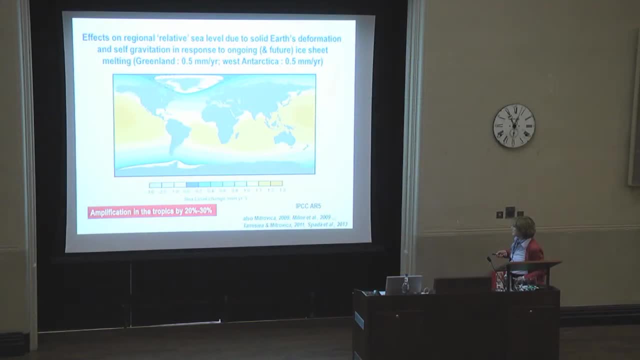 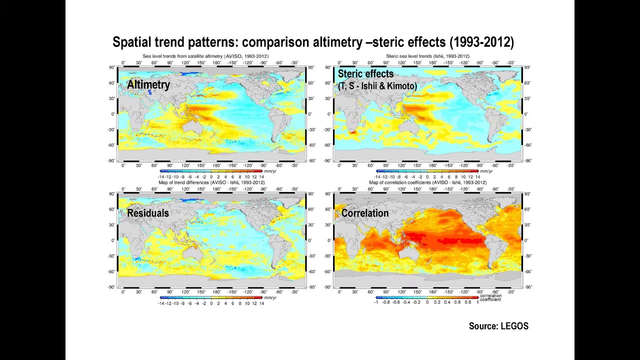 by the way, the same for West Antarctica, And this solid earth effect lead to an amplification in the tropics by 20% to 30%, as you can see on the map. So this is the result of the experiment that we 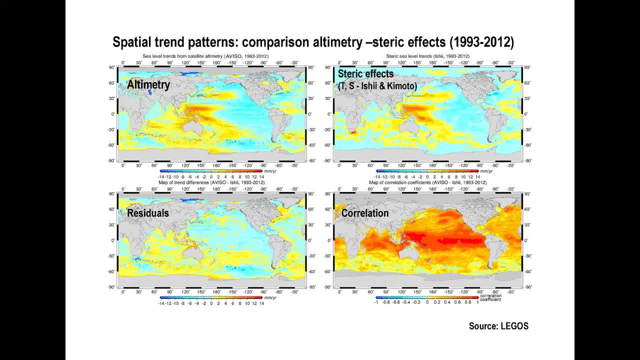 have done in the past years. So this is the result of the experiment that we have done with the Satellite Altimetry. Here's the steric effect. This is one data set, the JAMSTEC data set, Ishi, and. 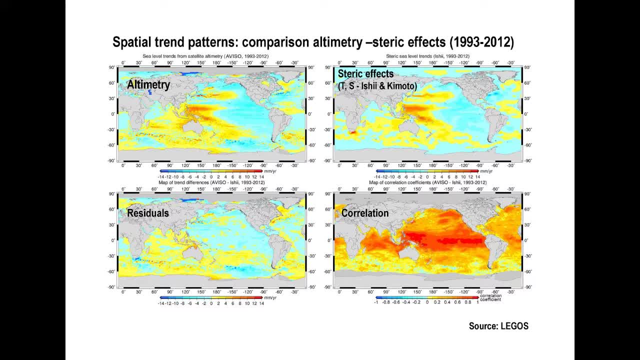 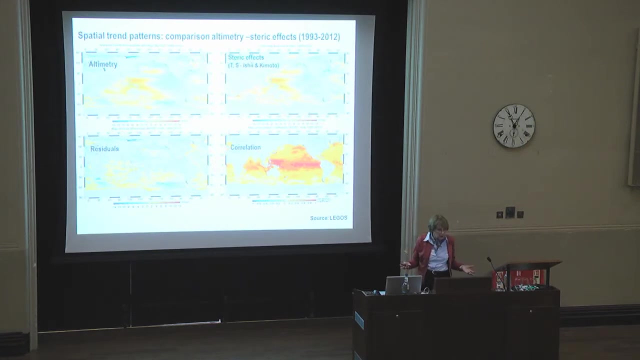 Kimoto. In both cases the global mean has been removed, So this is between minus two millimeters per year and plus two millimeters per year. So, and this is probably due to errors in the steric effect, The deep ocean. 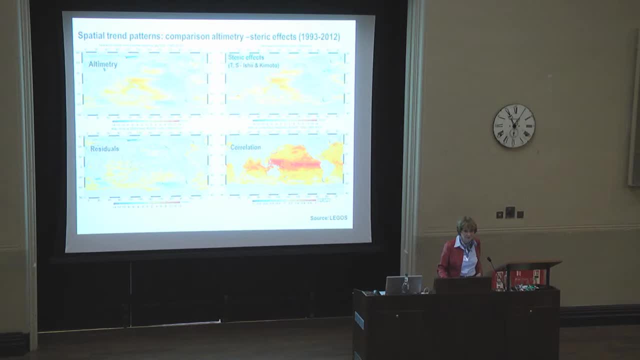 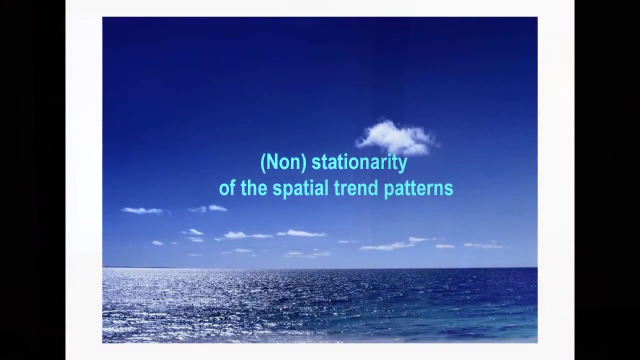 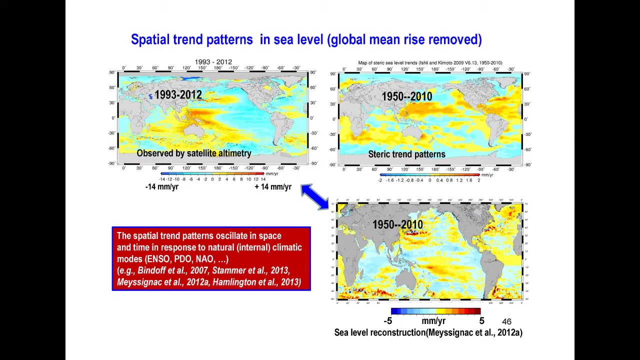 is impossible to detect the other signals And we have to work to reduce these errors, in particular for the altimetry data sets. So now the last few slides are about the non- stationary altimetry, The pattern we have observed. 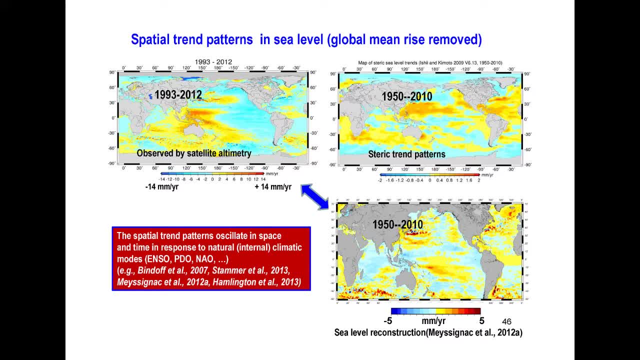 with satellite altimetry over the last two decades, are not stationary, permanent features, but they oscillate in time and space in response to natural climate modes, for example thermal expansion- Here you can see, because we have thermal expansion data for the last 50. 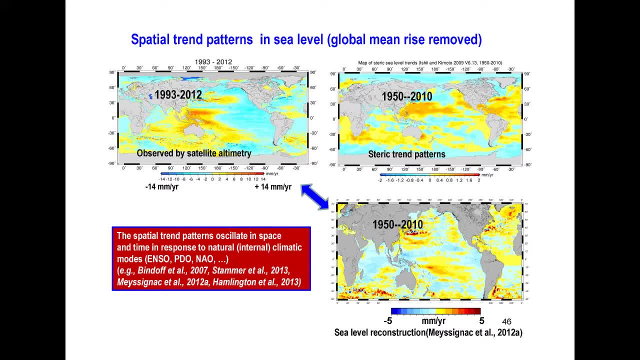 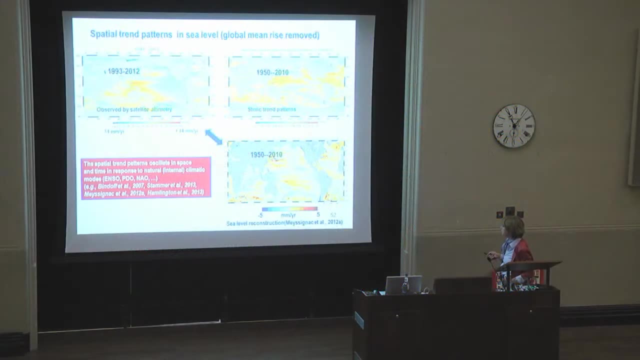 to 60 years. we can plot the special trend pattern from thermal expansion over a time span much longer than the altimetry time span, and the pattern are very different. It is also possible to use sea level reconstruction. In the recent years several 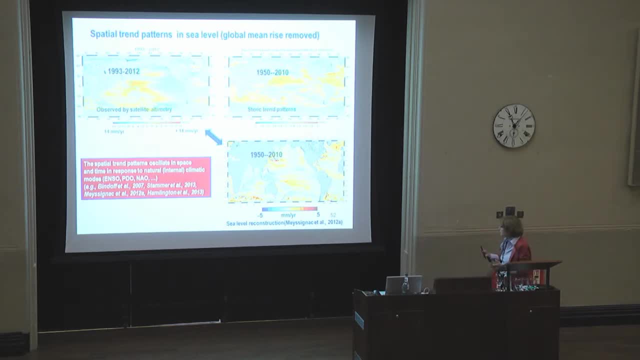 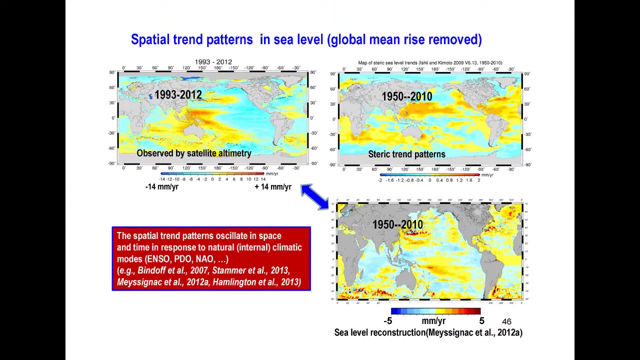 groups have tried to provide two- dimensional sea level data sets grids by combining tide gauge long and the dominant response, by combining tide gauge data with, for example, steric sea level data or output from ocean circulation models or satellite altimetry. 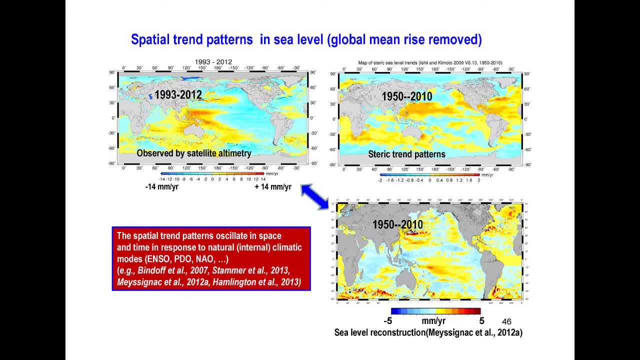 in order to get some two- dimensional time span longer than the altimetry era, And here is just an example. There are several other not mentioned here, but there are several studies by Hamilton Church and White Ray and Douglas and so 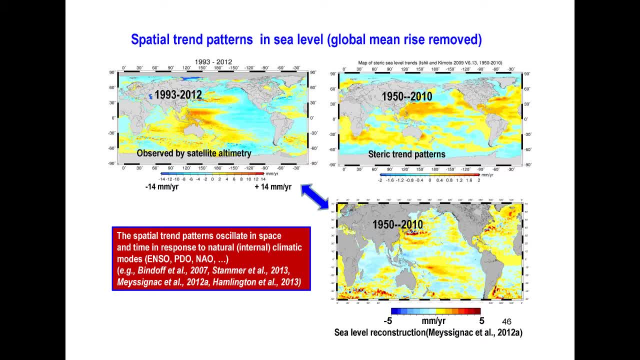 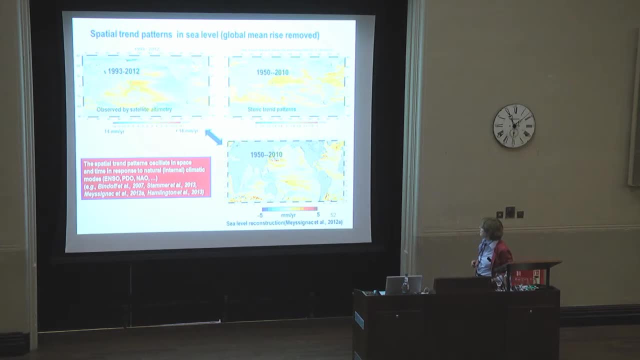 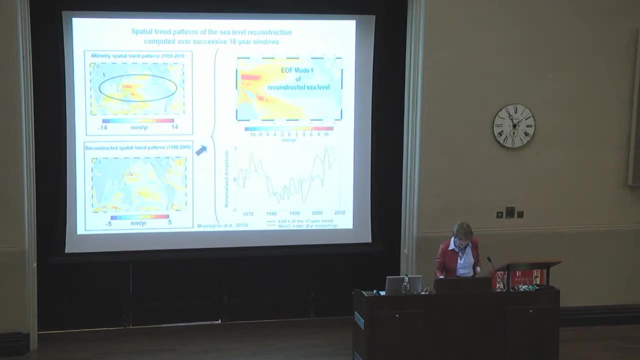 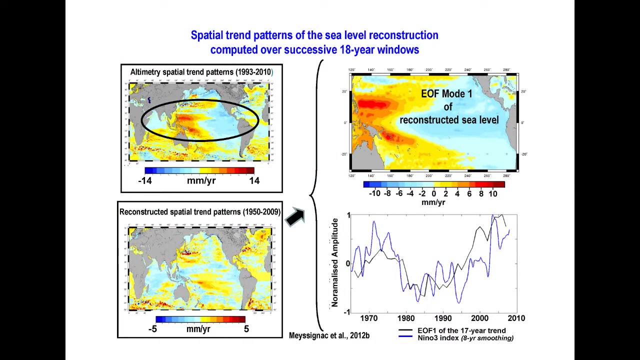 on who did this kind of spatial trend patterns over the 60-year period, the same as the thermal expansion pattern here, And you can see that they are very different from those reported during the altimetry era. And if we compute of this, 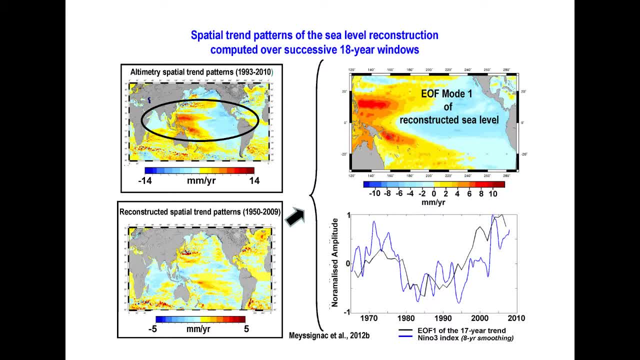 reconstruction. this is an example, the dominant mode here, the dominant mode of the AOF, reconstruction of the reconstructed sea level grids. what you can see is that the pattern seen is very similar to the decomposition, But what we see also is that the 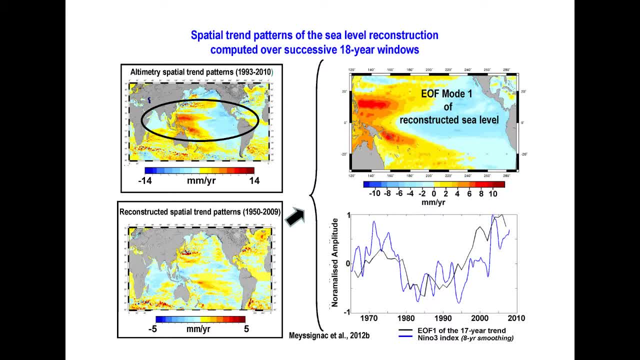 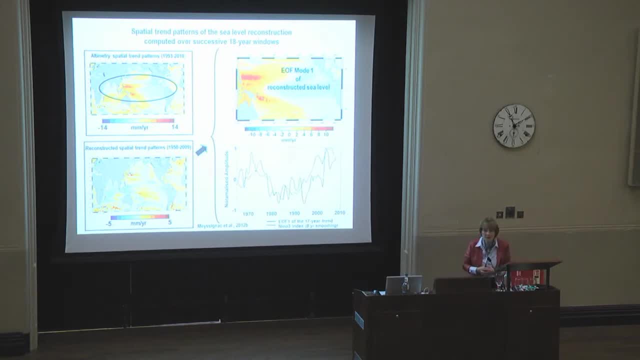 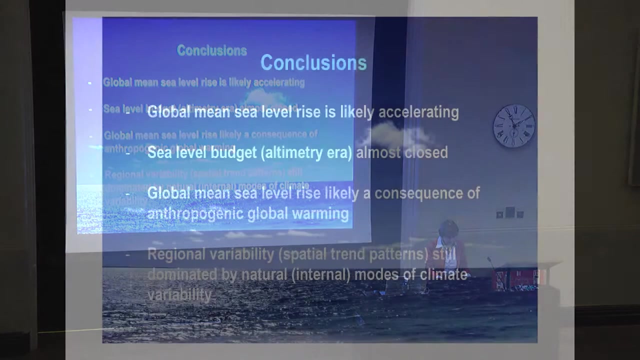 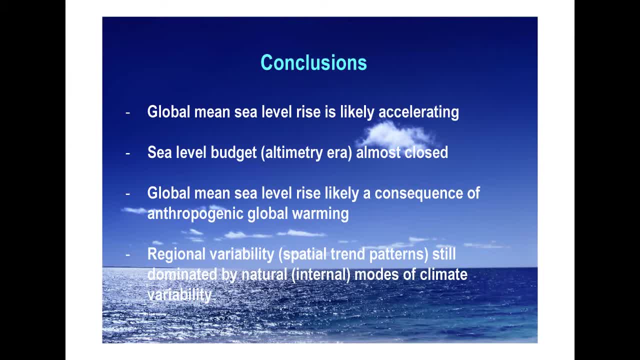 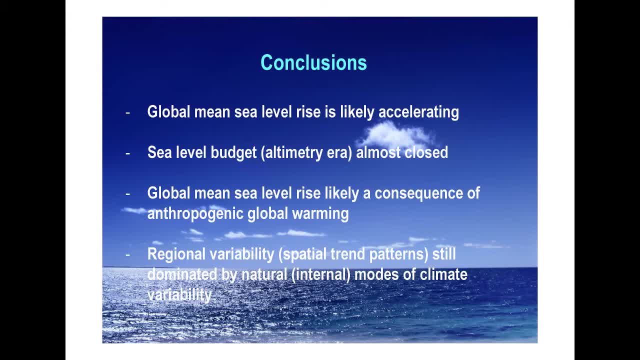 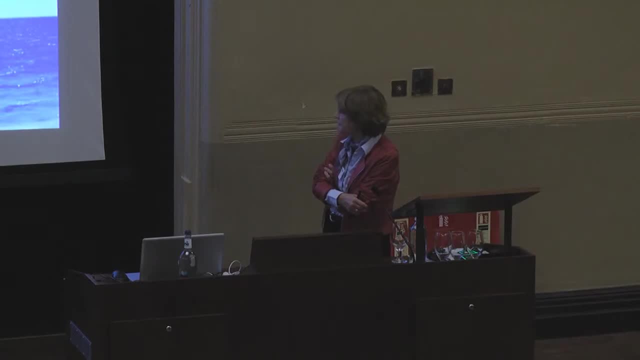 Maybe this conclusion doesn't come from my presentation, but mostly from, as also that the global sea level rise likely is a consequence of anthropogenic global warming. And another conclusion is that the regional variability as we have seen is still dominated by the natural internal modes of climate variability. 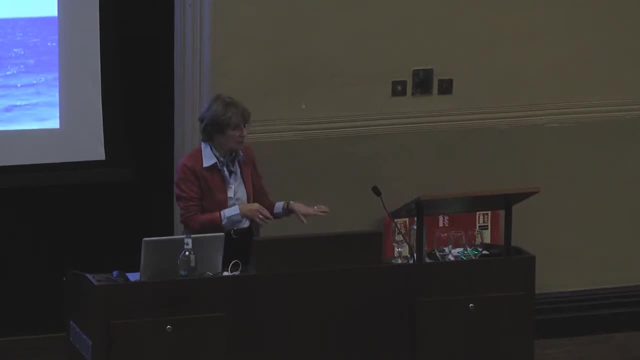 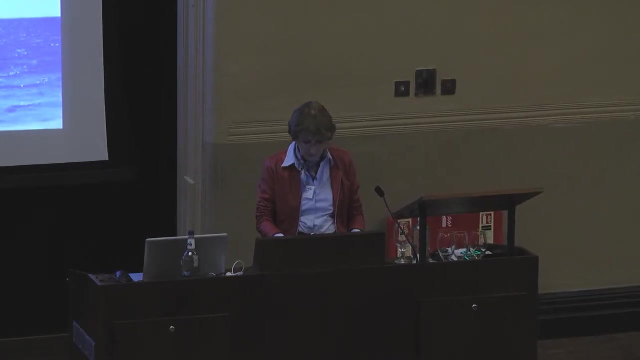 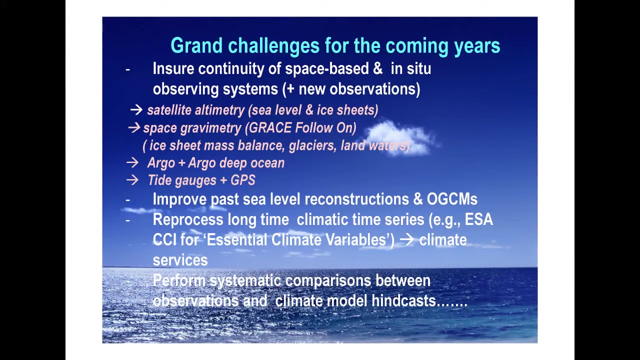 And today the signal-to-noise ratio is too low to really detect the anthropogenic signal. But maybe when the time span, time series, lengthen, maybe we will be able to do so. And this is my last slide. I think that the grand challenge in terms of observations for the coming decades coming 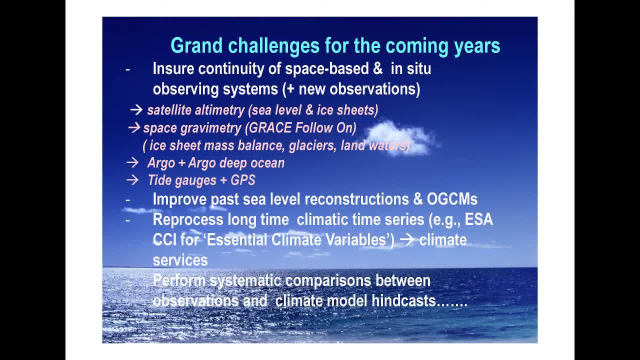 years, not decades, sorry. coming years is to ensure continuity of observation observing system, both space and in situ. We really need to To have long time series of altimeter satellites and this is not of use because we have as 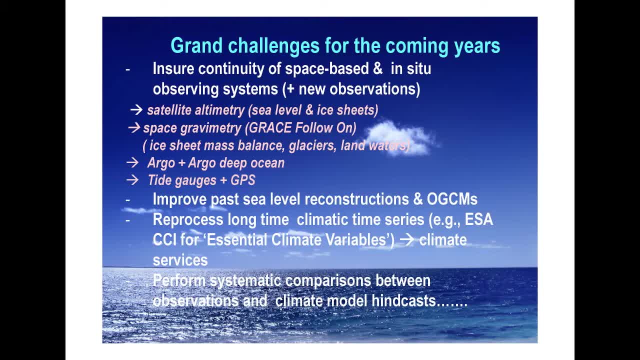 you know, we have to fight with the space agencies, And this is really not of use, first of all for sea level measurement, but also for the ice sheets. Another very important challenge is to ensure the continuity of gravimetry- space gravimetry. 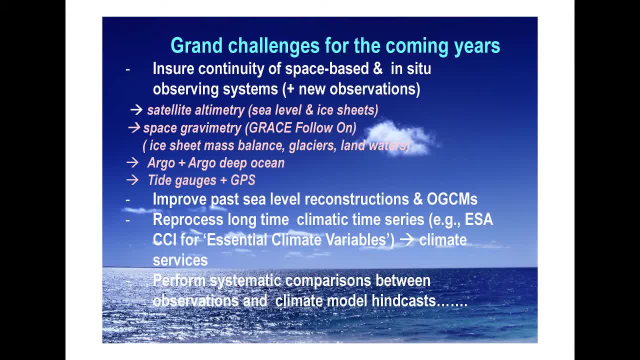 measurements. GRACE was launched for, I think, five years. It is now in orbit since 10 years, but it can die tomorrow And the next one, GRACE-Follow-On, will not be launched before 2017.. And very likely we will have a gap and I don't know how we will manage this. 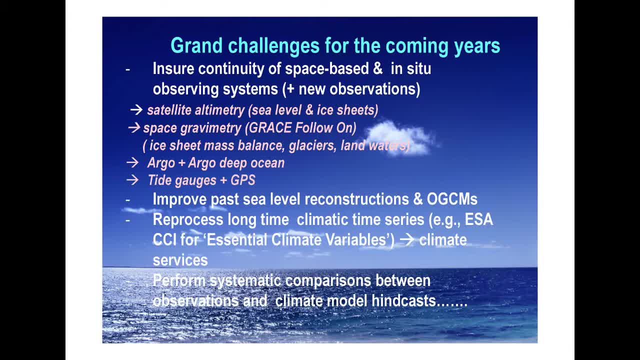 And GRACE is very important. Of course we have. also, We need continuity with Argo data and a new Argo-type system to measure the deep ocean contribution, And we also need high gauge with GPS for a lot of application, in particular for coastal. 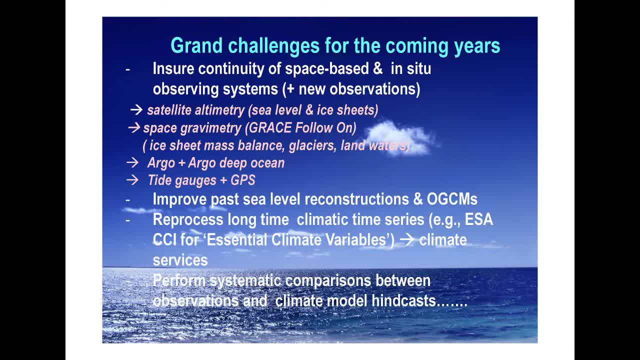 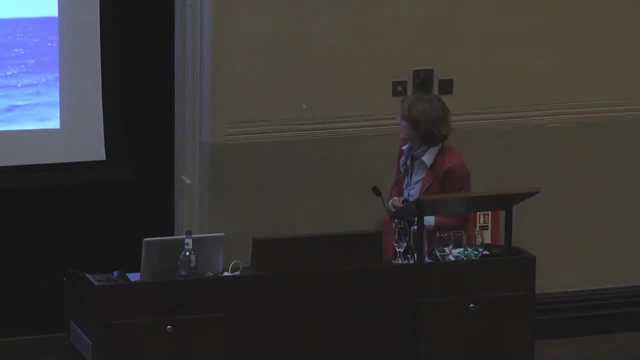 impacts of sea level rise. Okay, And I think what is also very important is to improve this past sea level reconstruction and also the model, And also the model. Okay, Thank you, Thank you, Thank you. Now the ocean reanalysis, I should say. 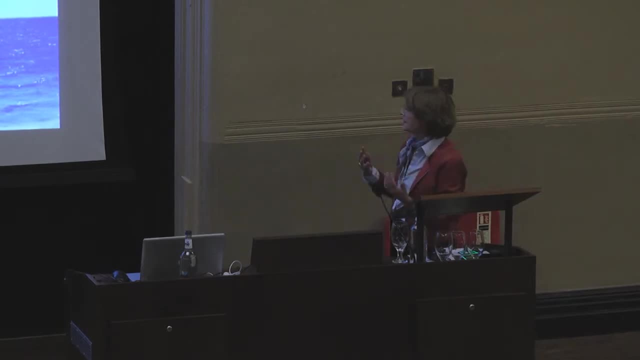 If we compare different reconstruction or different ocean reanalyses for the past few decades, there are big difference between the source of the data. So we have to understand why. and And finally, I will not talk about that because it is your- 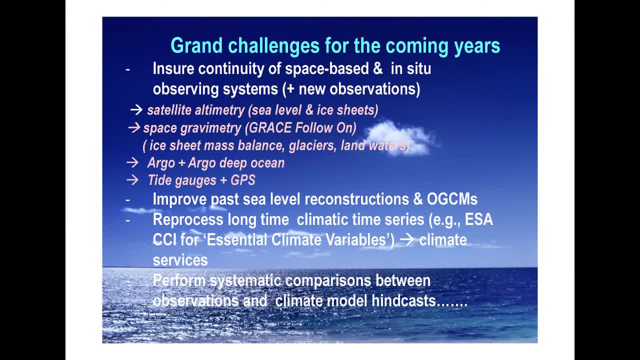 Yeah, Another important objective is to reprocess all data we have. I would like to give the example of the ESLA Climate Change Initiative, which is currently reprocessing data, space data, mostly space data for a number of essential climate variables. 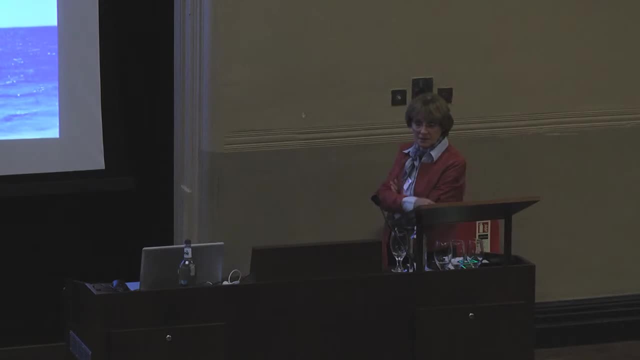 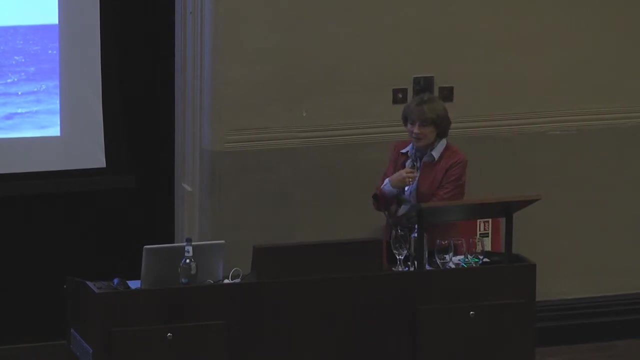 including sea level, but also ice sheets, glaciers, sea ice and so on. And this is very important because we know, at least at sea level, because I am more an expert in that domain- that there are still errors, in particular, on the regional scale. 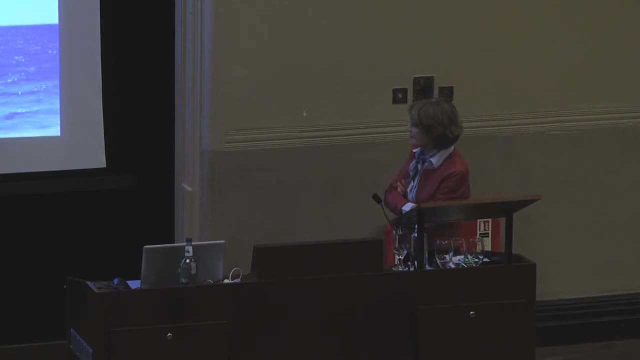 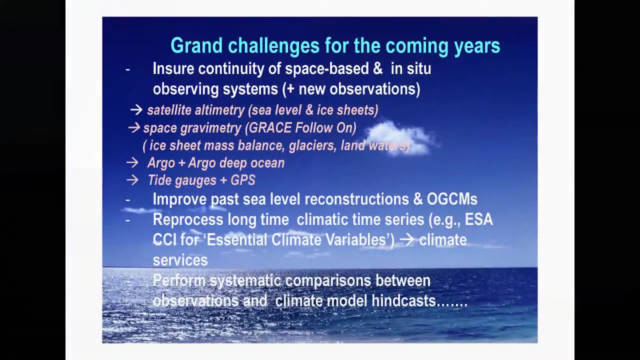 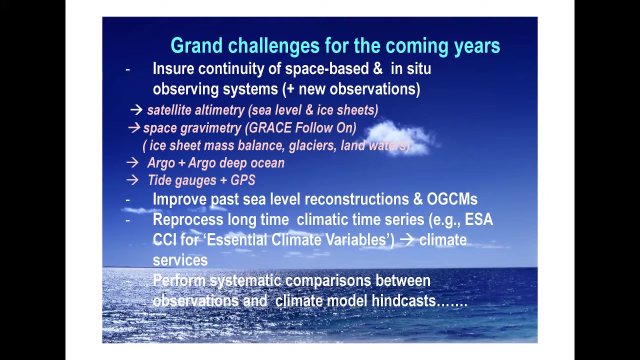 And if you want to detect the solid dust processes, we need to remove these errors. So this is another fascinating talking point objective. I think we have to work more on comparison between observation and climate model outputs, or hindcasts. I think some work is done, but not enough.